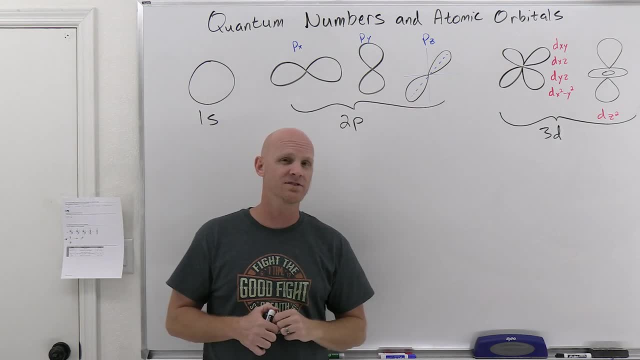 turns out there's also g orbitals and h orbitals that you probably don't know about, but there's a lot of them in this course, so let's dive into this. so let's dive into this. so here i've got diagrams probably won't talk about in this class because we don't actually have any, uh, stable elements that. 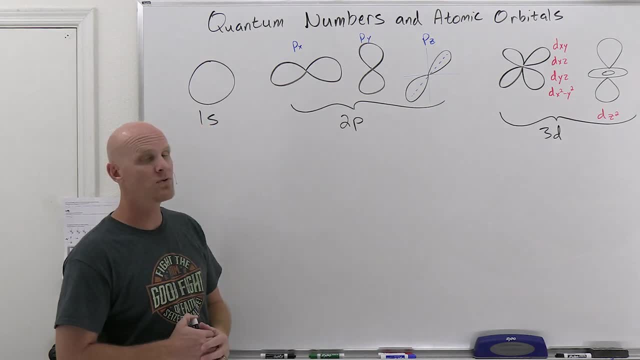 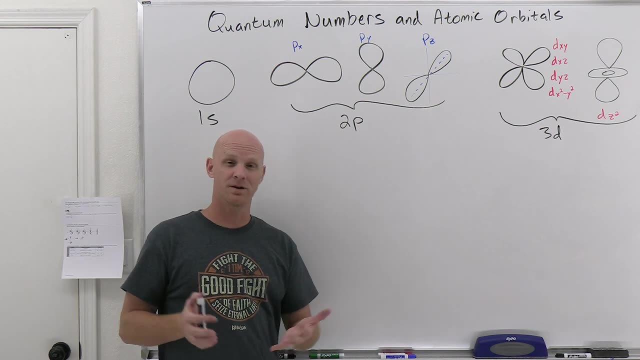 have electrons in them normally, so, uh, but we'll talk about the f orbitals. but turns out the shapes of the f orbitals are more complex that i can't draw them for one. but you typically won't even find illustrations of them in your textbook. but if you google them you will find shapes for them. 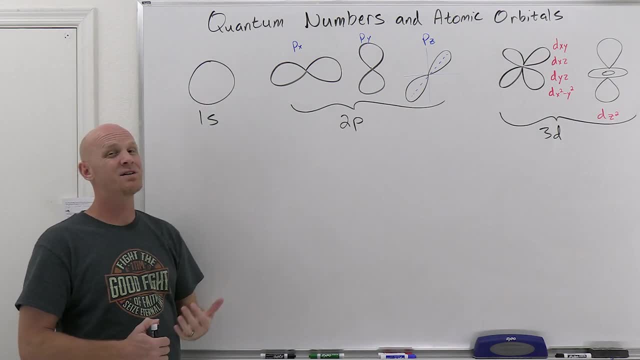 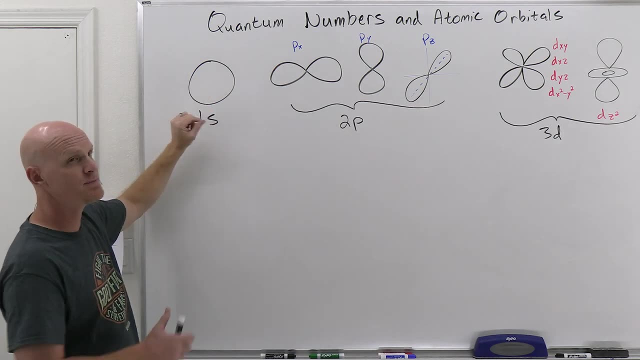 so it turns out where these shapes come from. so it turns out they are mathematical, three-dimensional mathematical equations that we call wave functions, and this is just the three-dimensional graph. so this is not too dimensional. think of this as a three-dimensional sphere. we like to think of the p orbitals as being. 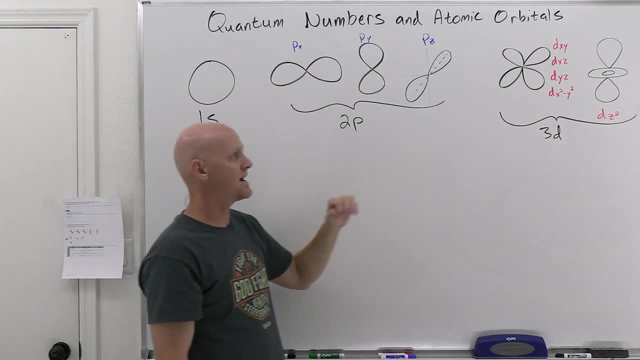 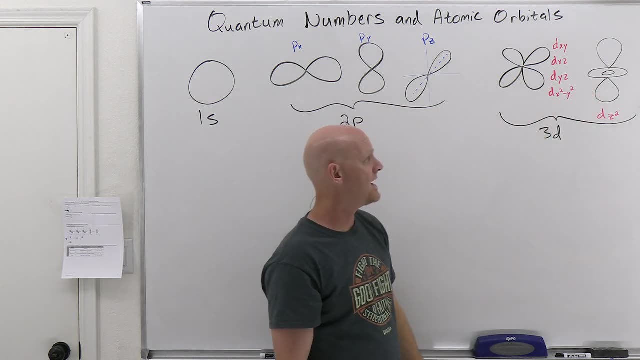 dumbbell shaped, but again they're three-dimensional in space. and then the d orbitals are either going to be four-leaf clover shaped or they're going to have this kind of toroidal shape. we say, and it turns out that four. there turns out there's just a single s orbital, there are three p orbitals. 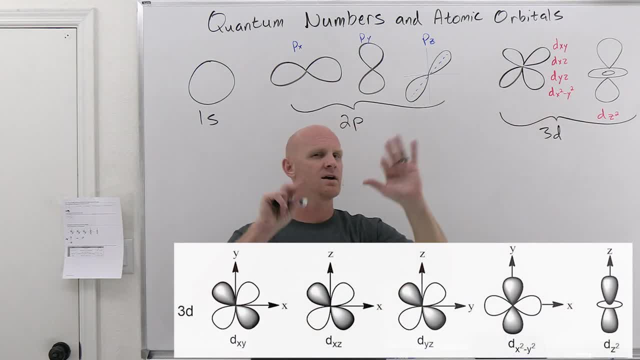 but there are five d orbitals, and then there are seven f orbitals, and if you see the trend, so again one s orbital, three p orbitals, five d orbitals, seven f orbitals, nine g orbitals, if we cared, eleven h orbitals, if we cared they. 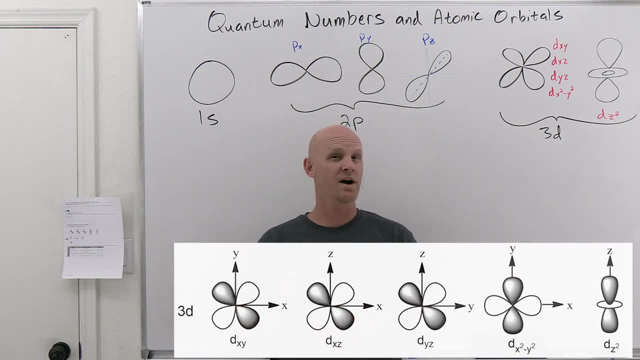 count on the odd numbers. uh, we'll see why when we get to quantum numbers. why exactly that is so, but you should know it well. for the d orbitals, i just got lazy and didn't draw them all but four out of the five turns out. they get labeled dxy, dxz, dyz, dx squared minus y squared. four out of. 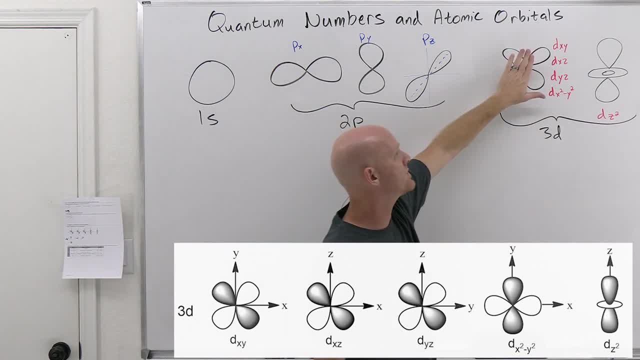 the five look like a four leaf clover. what's going to be different, though, is how they're oriented on, you know, in space. so dxy, it turns out, is in the xy plane, dxz in the xz plane, dyz is in the yz plane. 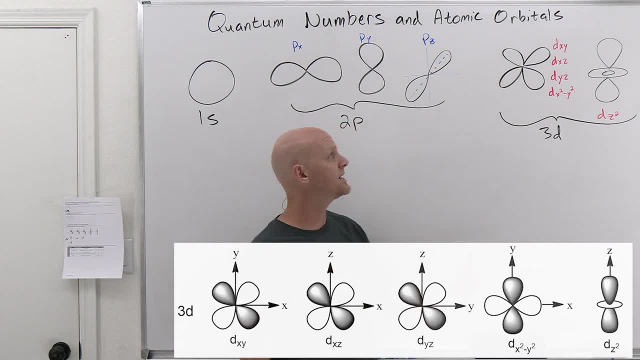 so, and then dx squared minus y squared, it turns out, is also in the xy plane, but whereas dxy is in between the x and y axes, dx squared minus y squared be right on the x and y axes. and uh, then dz squared here. so it turns out the big lobes here are going to be on the z axis. and then 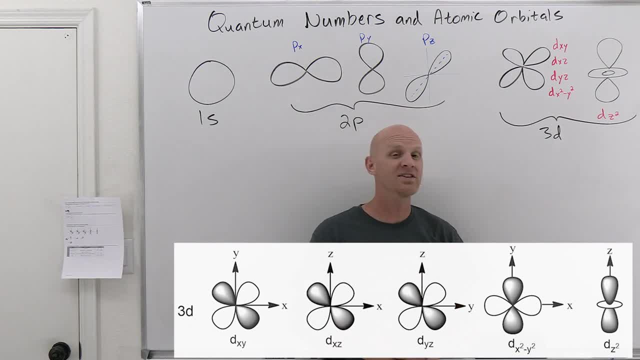 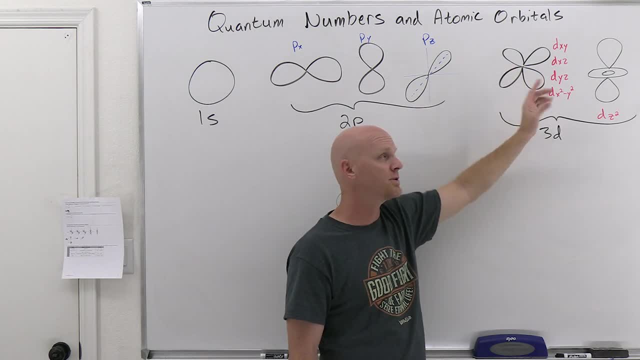 this lovely circular portion- the donut portion, if you will- is going to be in the xy plane, cool. so i want to distinguish that. but i want you to realize that, even though i'm lazy, there are five d orbitals, even though i only drew two of them here. so. but these four lobes represent a single orbital. 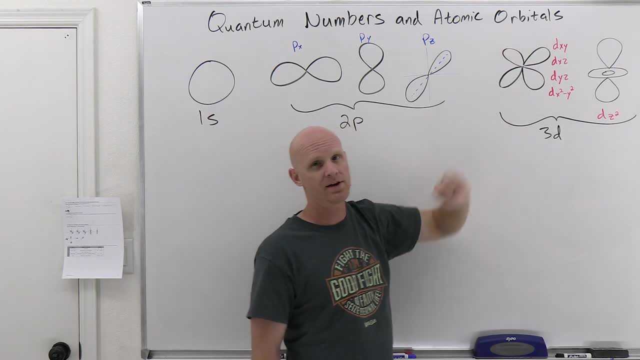 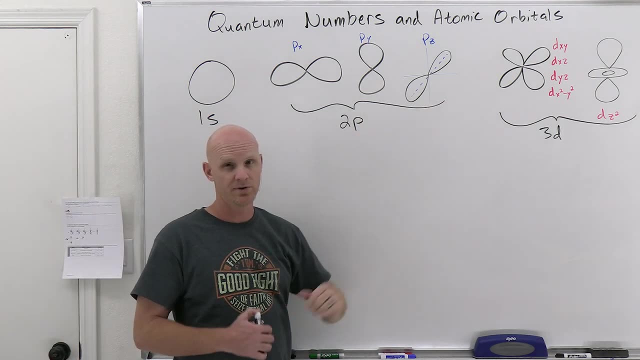 and again. you could hold a maximum of two electrons in an orbital like that. okay, one thing you should know is that i'm giving you the most basic version of each of these orbitals, so, the first time you'll ever, the lowest shell number that actually has an s orbital is the. 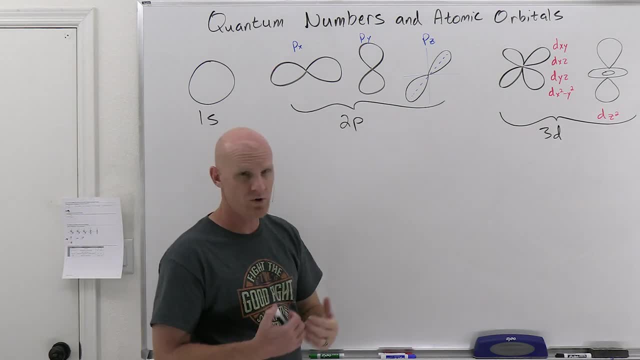 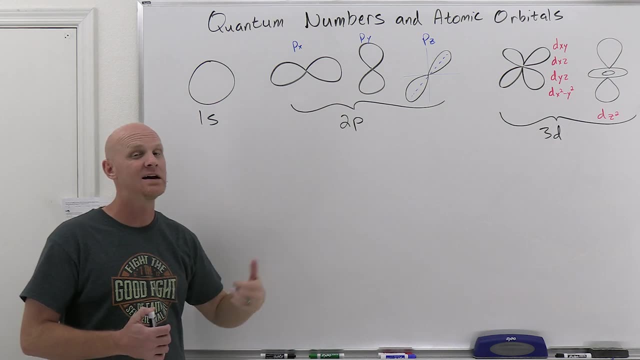 first shell, the lowest shell number that has p orbitals is the second shell, the lowest shell. but as you go higher and higher it actually turns out that those same type of orbitals that you encounter again get a little more complex, a little more complicated. so, like when you go to 2s, it's a 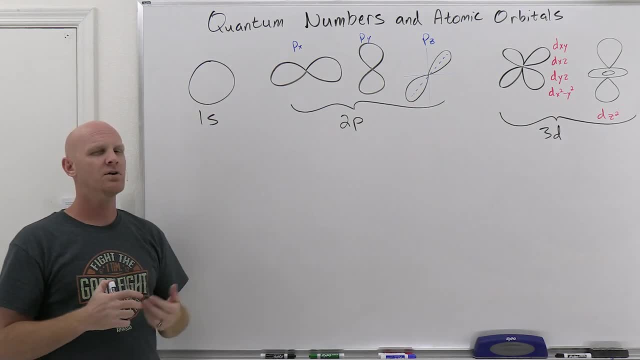 bigger sphere, okay, but it also turns out has what's called a node in it, and it's kind of like, you know, putting a softball inside a basketball, so to speak, and the air space in the middle is going to be a node where you don't find the electrons, and you could find them in the softball. 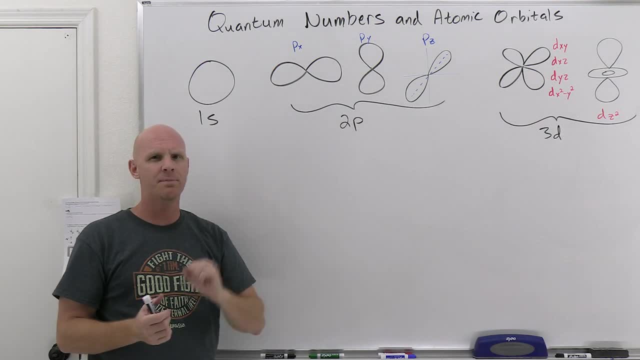 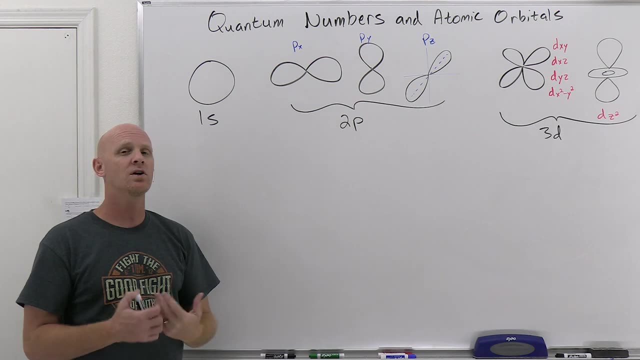 region in the middle or you could find in the outer region, but there's a hollow gap in the middle that you don't find them. it's really weird. and they get more complex as you go up. as you go up to like 3s you'd have two of those nodes- we call them radial nodes and stuff and not super important at. 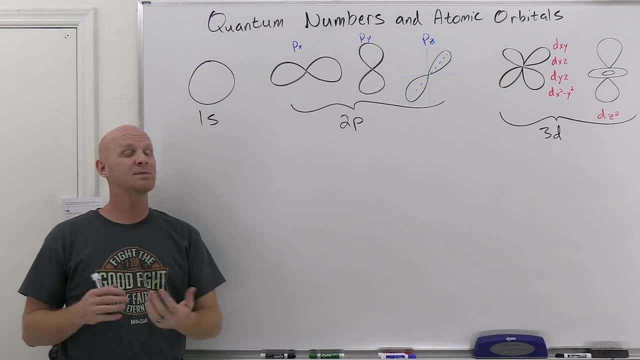 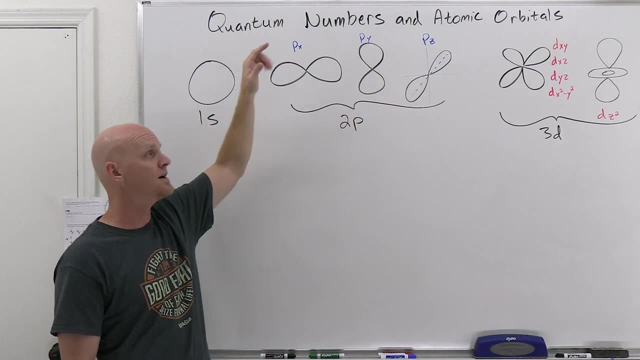 this level. so. but if you take a more advanced, like physical chemistry class, or if you're taking maybe a majors class, they might go through something like that. so. but the same thing happens with the p orbitals and d orbitals. if you go from 2p, if you go and talk about the 3p, these orbitals get bigger. 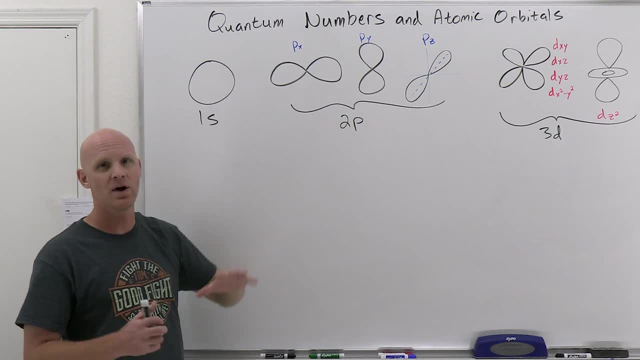 but again they have these radial nodes incorporated into their shapes and stuff. so i'm not going to say any more than what i just said about them. i just want you to realize that there are more shapes when you get to the higher shell versions of these same types of orbitals. 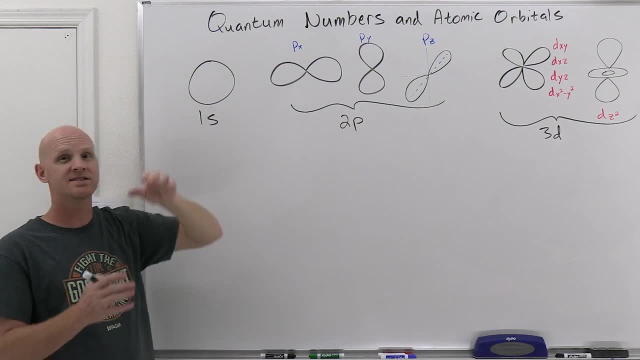 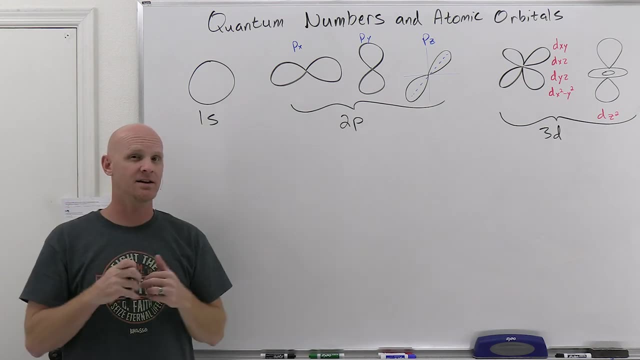 all right now. one thing i did say, though, is that as you go from like 1s to 2s to 3s, they get bigger, and, if you recall, then that means the electrons that are going to occupy them get higher energy, because, again, the closer an electron is to the nucleus, the lower its 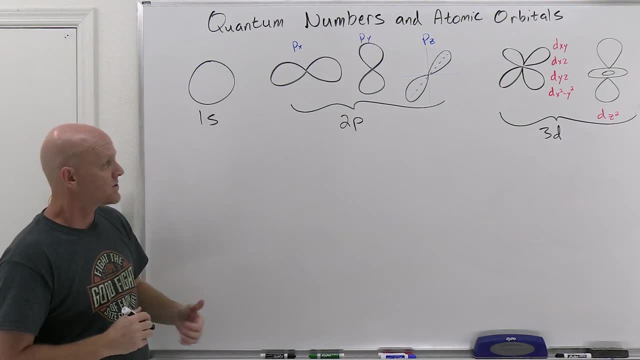 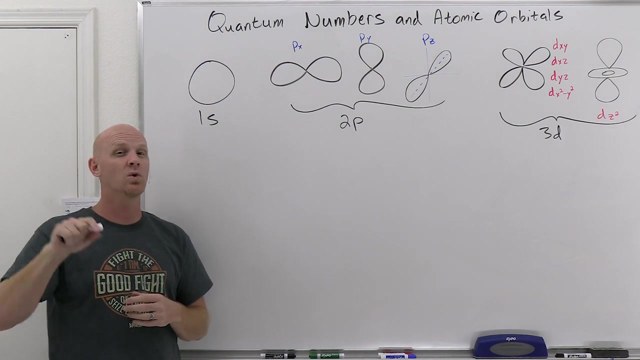 energy, as we learned a couple lessons ago. so it turns out, then, that the lower the shell number, the smaller the orbitals and the lower the energy, the electrons that are in those orbitals. so you can see here that the nucleus is already 3d and the orbital is just in the middle. we 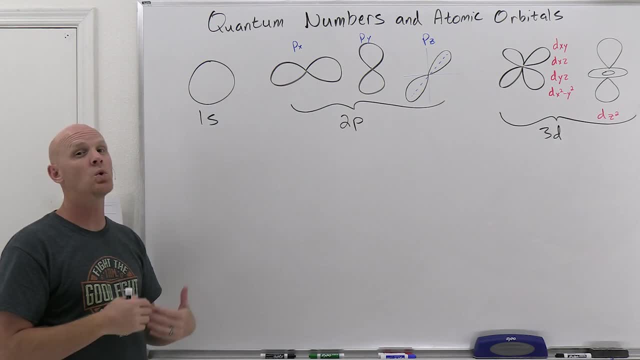 can see here that it's actually a 2d orbital that gets double times the energy, and so, back when we studied the bohr model of the atom, bohr thought electrons went around the nucleus in these two-dimensional circular orbits. what's really true we find out, though, is that it's actually 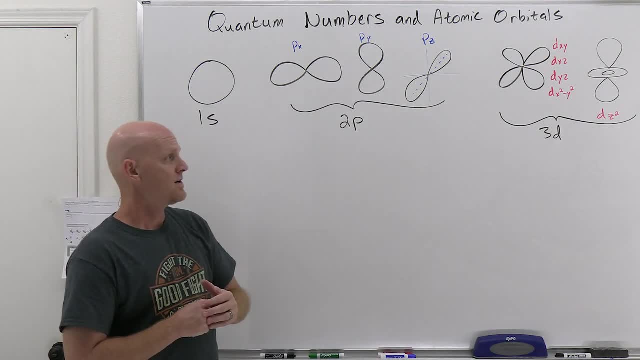 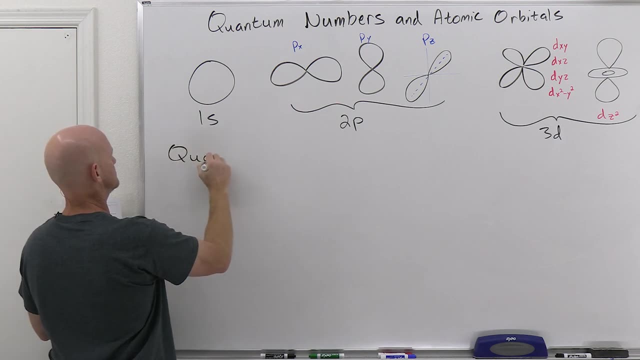 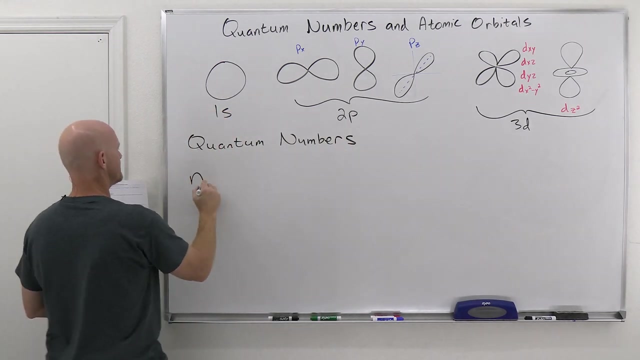 these three-dimensional orbitals, that electrons actually live and they have a wave-like property that bohr really didn't take into account. lovely quantum numbers, And it turns out there are four of them. There's n, there's l, there's m sub. 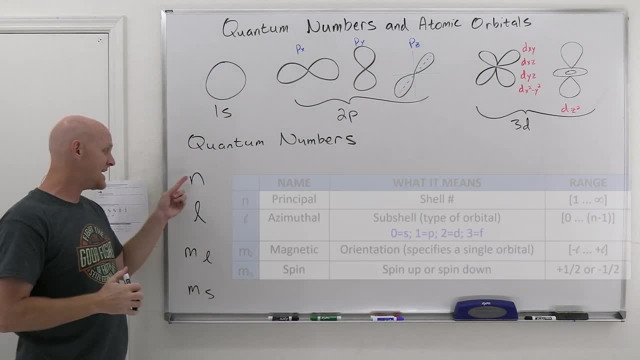 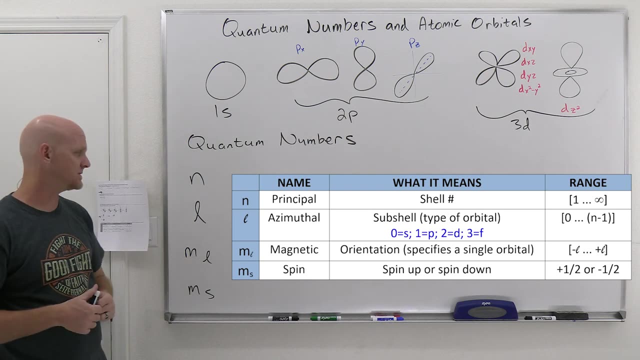 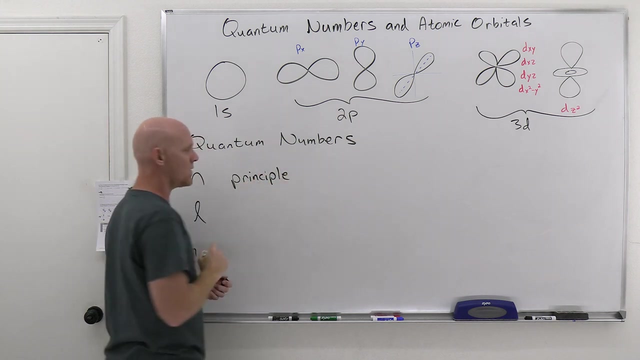 l and there's m sub s. You should know the name of each of these quantum numbers, You should know what they tell you and you should know what range of values are possible. So if we look at n first, so n is going to tell you, or n is called, I should say, the principal quantum number And it's 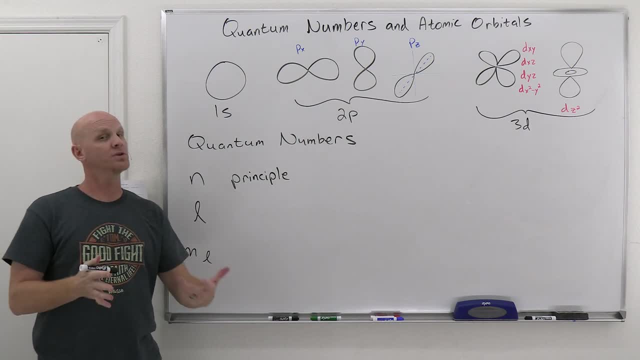 going to tell you what shell its electron is found in. what shell the orbital, I guess, really is in that the electron is found in, And in this case you have, like, the first shell, the second shell, the third shell, And again these are the same n values that correspond to the Bohr model of atom. 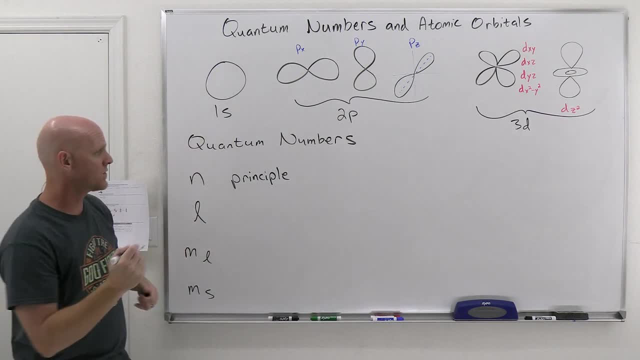 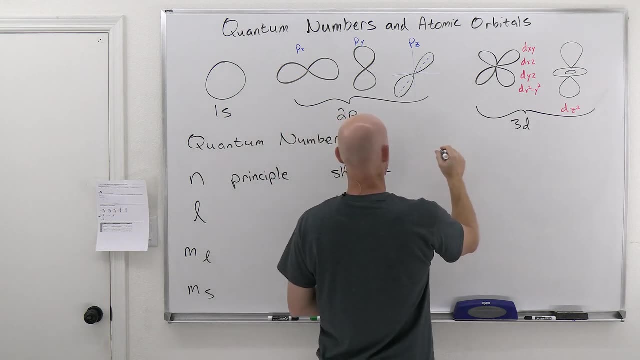 like the first orbit, the second orbit, the third orbit, according to Mr Bohr there. So in this case we're going to say that they give you the shell number And if we look at the range of values that are possible, so in this case the lowest shell is shell number one, And then it 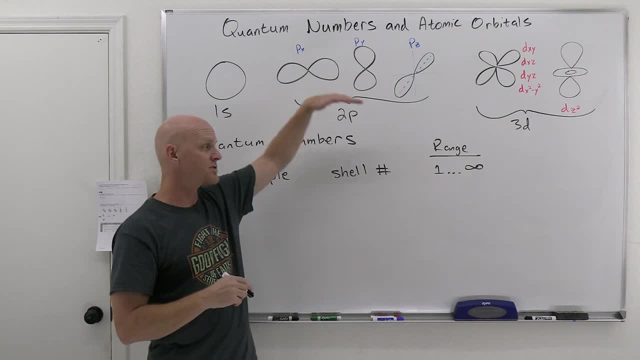 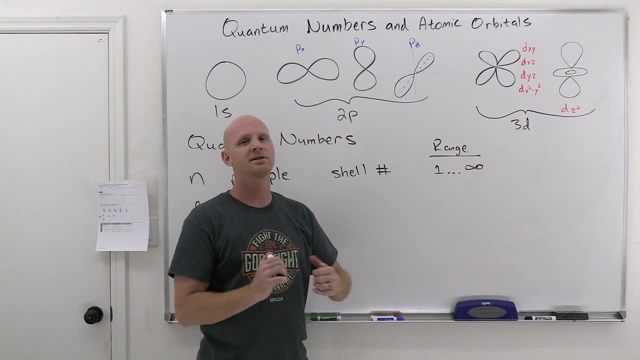 turns out. just like with Bohr's orbits could go up to the infinitieth orbit, so can the shells: the first shell all the way up to infinity. So you should know, though, that in the ground state we only have atoms with electrons up to like the seventh shell, But again, we can verify that the 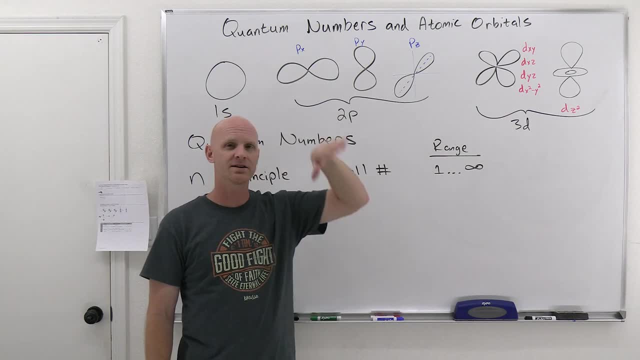 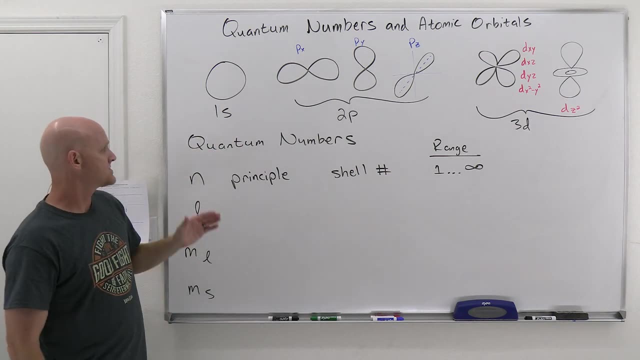 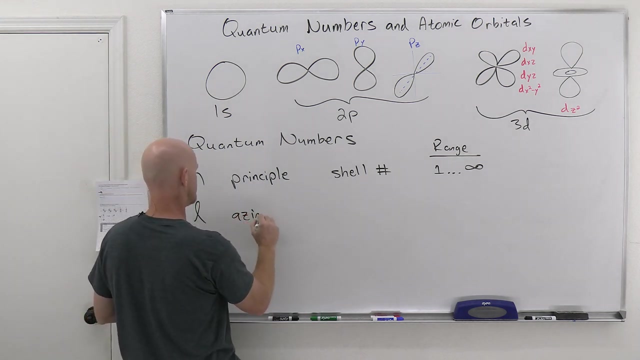 additional shells do indeed exist by, you know, looking at different electron transitions, where electrons are actually promoted up into those higher energy orbitals. Okay, so that's our principal quantum number. Next on the list is L. here, And L is often referred to as our azimuthal quantum number. So, and your azimuthal quantum? 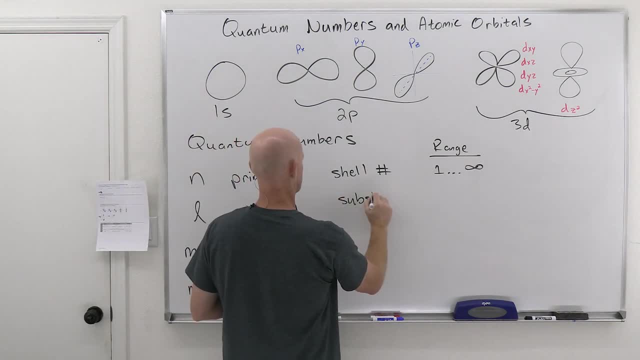 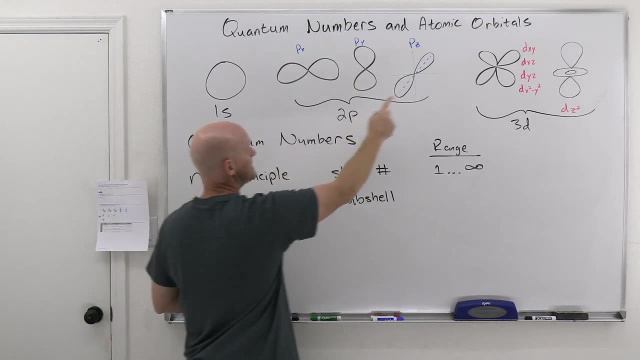 number is going to tell you the subshell. So- and you can kind of think of this as a code here- So the subshell in this case could be S, P, D or F or again technically, G or H, but you're never. 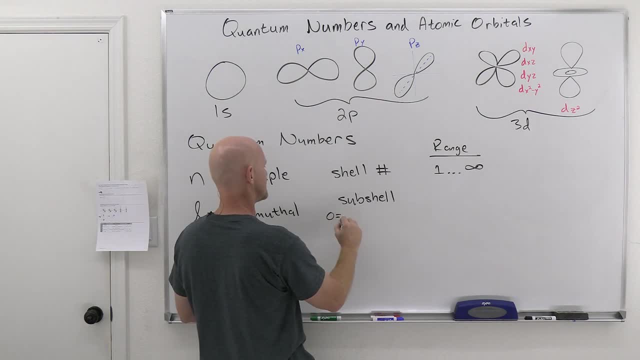 going to get it. So S, P, D or F, and it's a code here. So zero is going to tell you that it's an. let's put this in blue actually, just like it is on your study guide. 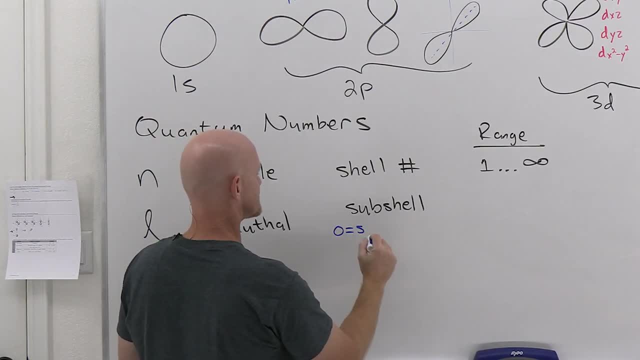 So when L equals zero, a value of zero, that tells you you're an S subshell. When L equals one, it tells you you're in a P subshell. When L equals two, it tells you you're in a D subshell. And when 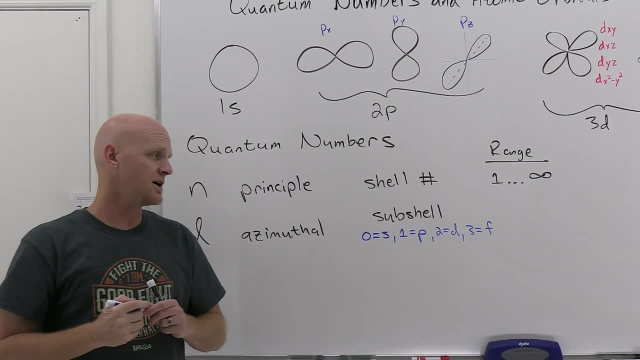 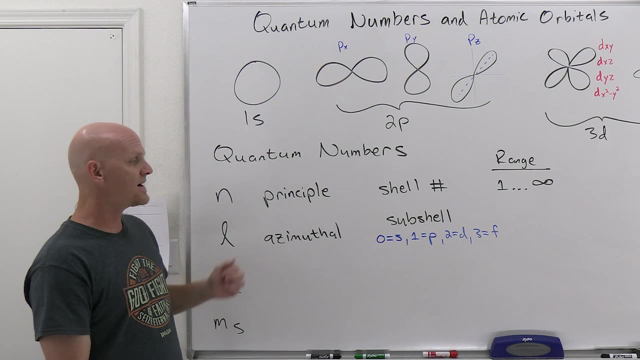 L equals three. it tells you you're in an F subshell. So these quantum numbers are going to describe, and I say U, but it's really describing where an electron is found in an atom. And so if zero, you're supposed to know, oh, that electron is in an S orbital somewhere. So if I say L equals, 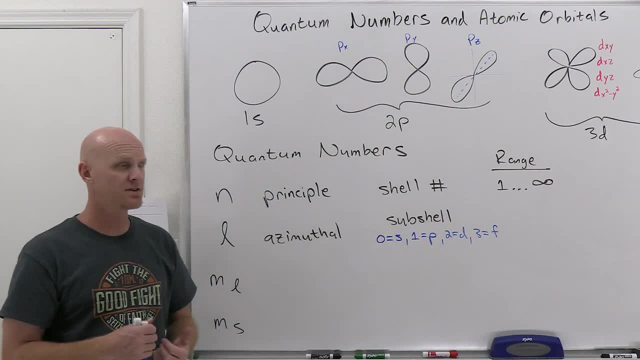 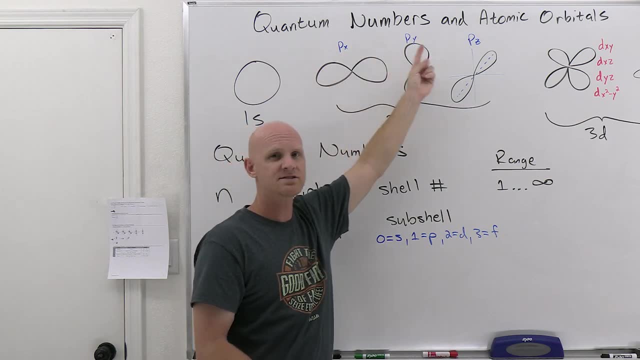 one you're supposed to know. oh, that electron's found in a P orbital somewhere And we call it the P subshell, because in any P subshell there are actually three P orbitals: one on the X axis, one on the Y axis, one on the Z axis, And when L equals one, the electron that has that value of L. 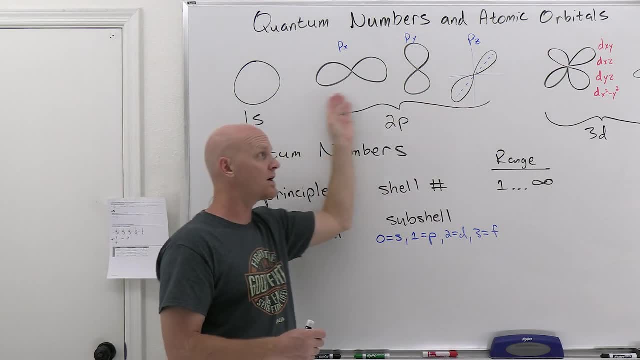 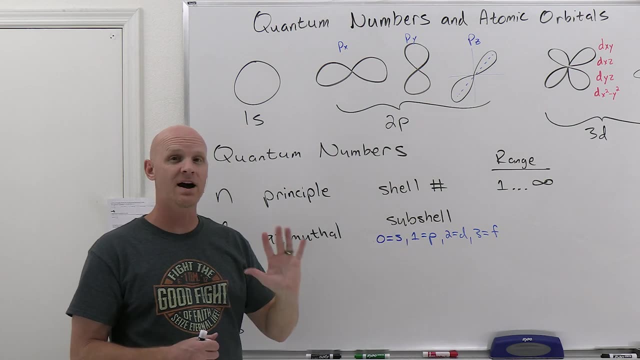 equals one has an electron in one of those three orbitals and somewhere in the entire P subshell. All right. When L equals two, that electron is in the D subshell, one of the five D orbitals. And when L equals three, 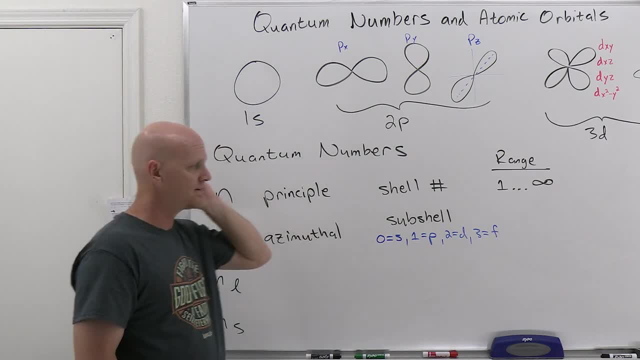 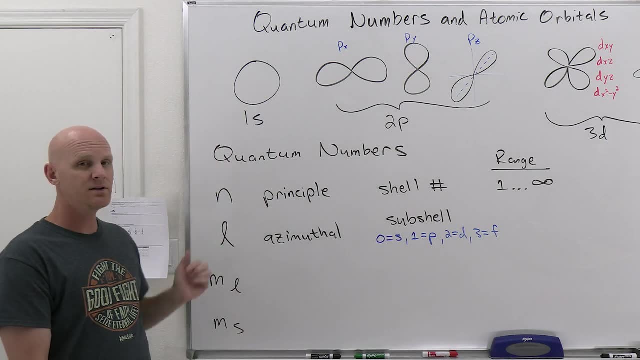 that electron's in the F subshell, one of the seven F orbitals. All right, If we look at range of values here. so we like to define the range of values for L in terms of N. So and it turns out: 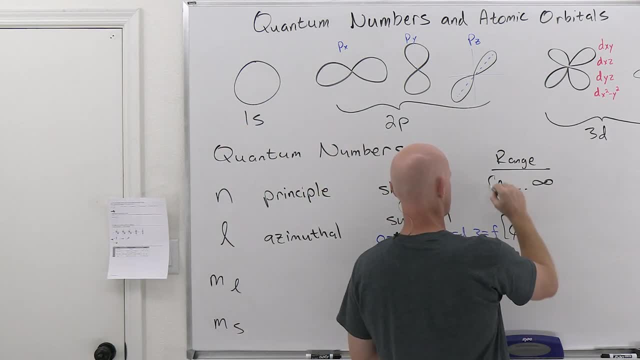 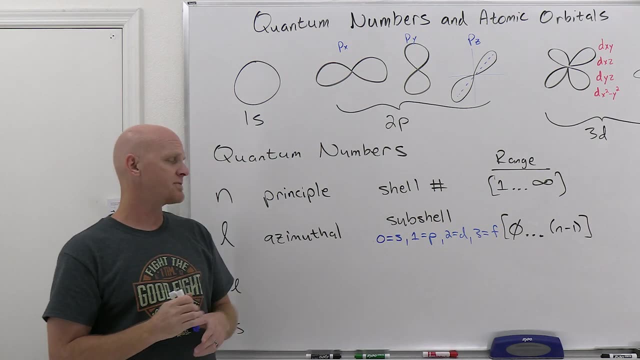 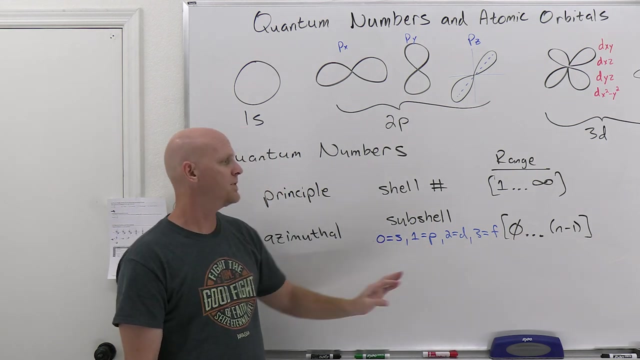 it can start from a minimum value of zero up to a maximum of N minus one. So we'll see the profound here in a sec. So, but in this case- so notice- the lowest value could have a zero. We saw that. but the highest value it takes depends on what shell you're in. If you're in shell number one, 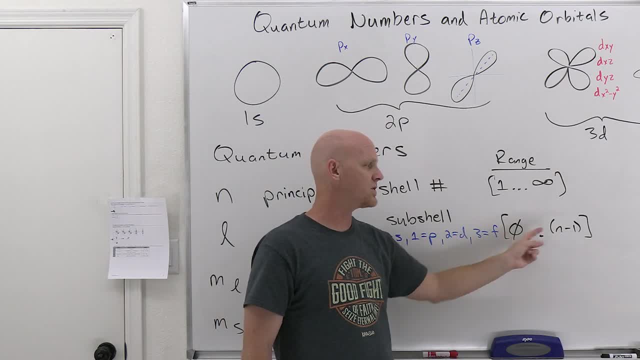 ie, N equals one. well, one minus one is zero, and zero up to zero means it's the only values it can take is zero. And so here, from zero to N minus one, all the integer values in between, and I should have said that up here as well. your range for the shell number is any integer value. 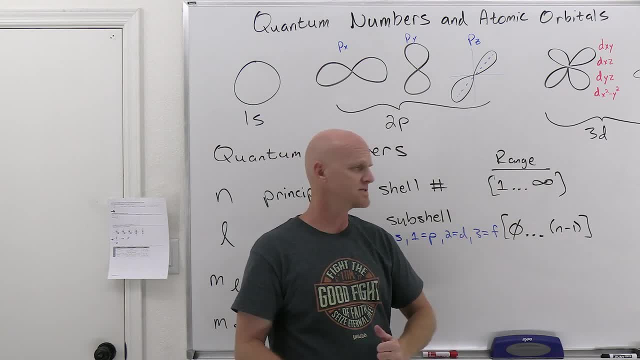 from one to infinity. So one, two, three, four, but not like 3.476.. So all integer values, Cool. So, if you're in the second shell, N equals two. well, two minus one is one, And so 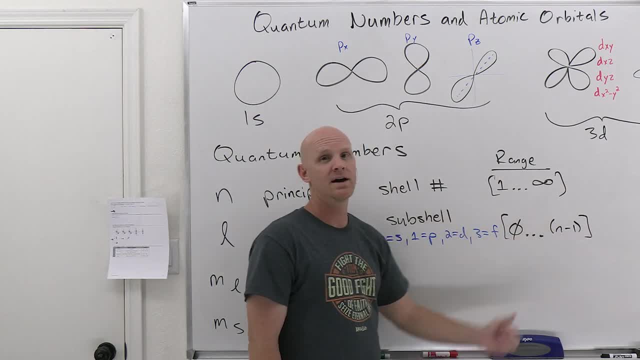 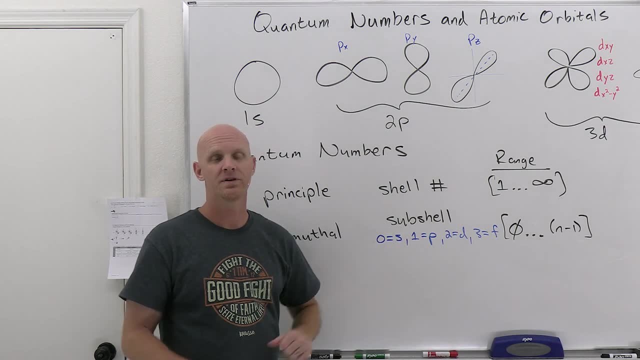 it can take any integers from zero up to one, And so in the second shell it could be zero or it could be one, And in the second shell there are S and P orbitals only. In the first shell there were only S orbitals because the only value L could take was zero. In the third shell, 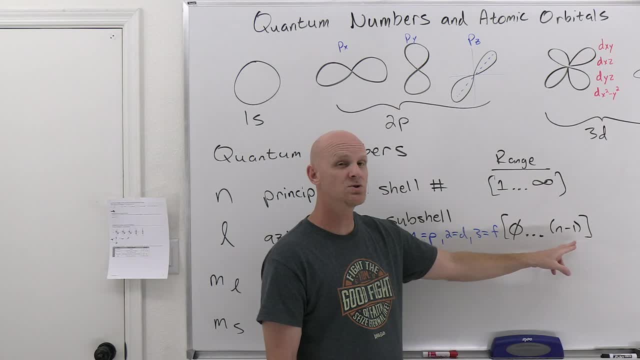 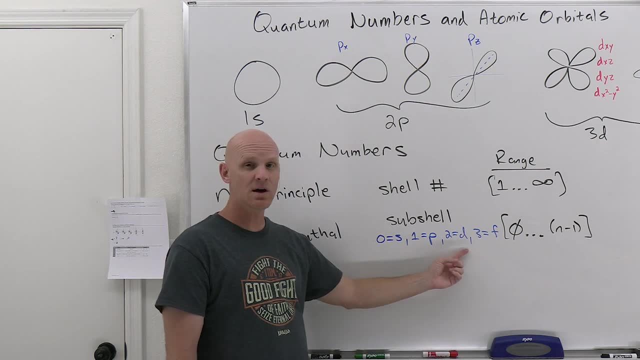 you've got zero up to three minus one, zero up to two. So zero one and two and zero two mean that in the third shell there are going to be S, P and D subshells, ie S, P and D. 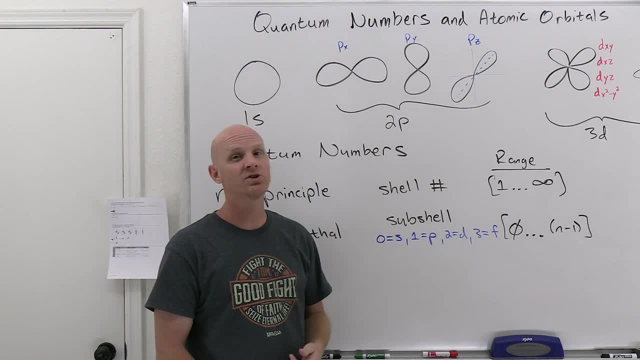 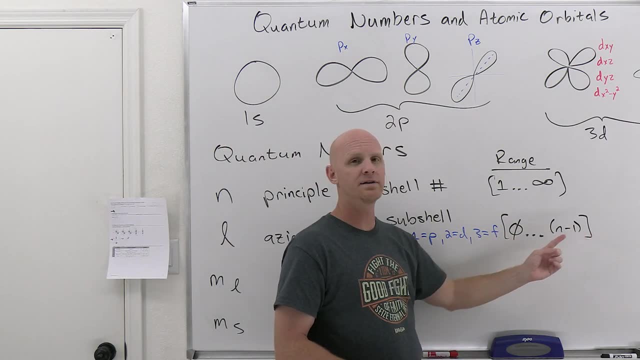 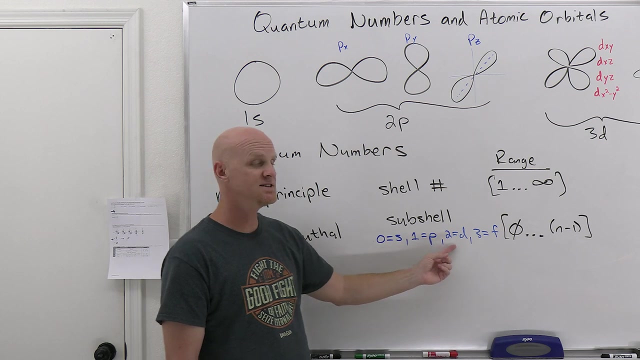 orbitals, And so every time you go to a higher shell you get something new. it turns out In the fourth shell you've got L taking on values of zero up to four minus one, ie zero to three. So zero one, two and three, Because in the fourth shell there are S, P, D and F subshells. 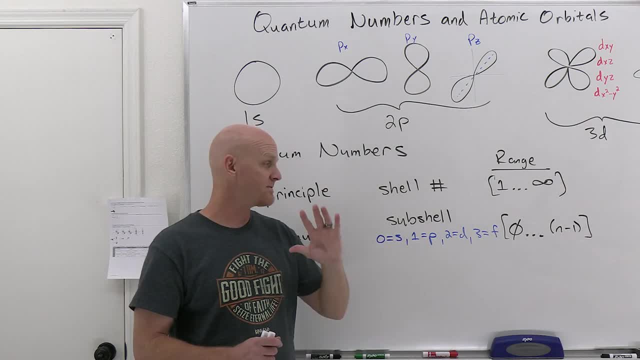 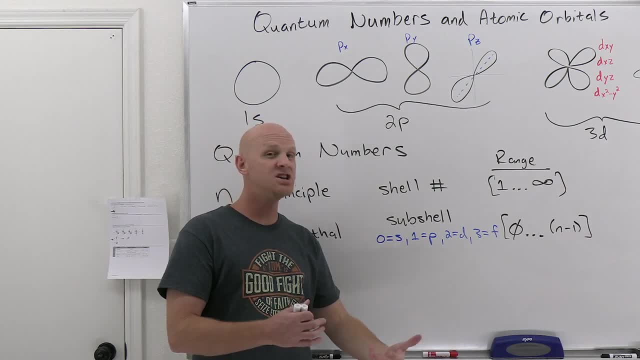 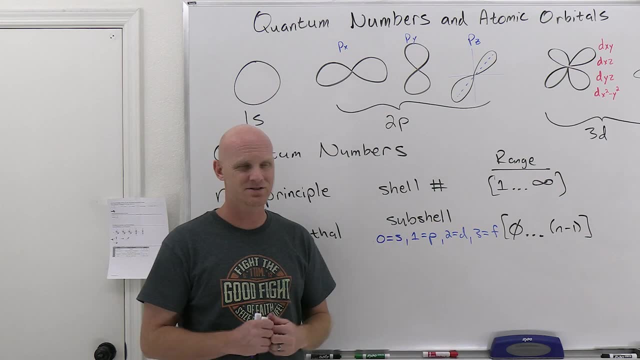 the fifth shell. that's where you'd actually encounter the G orbitals, the G subshell. But again, no stable elements actually put any electrons in there and we don't ever talk about them. So I just bring it up, just so you can follow the pattern here. So all you got to know. 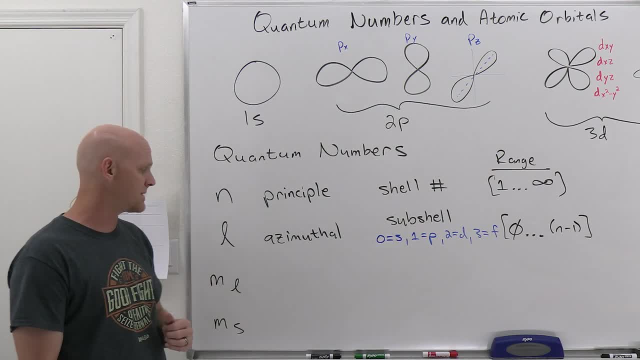 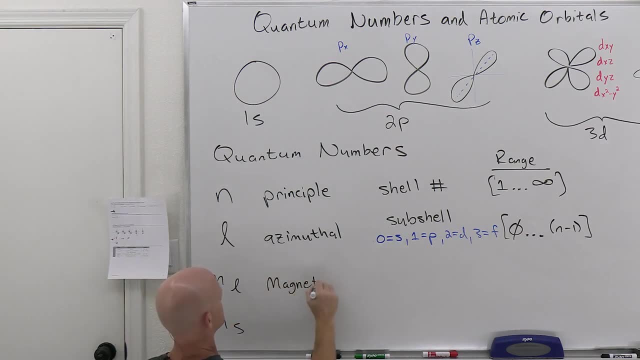 is up to F orbitals, Cool, But that's how the azimuthal quantum number works. And so, moving on to M sub L, and M sub L is our magnetic quantum number. So, and in this case it's going to tell, 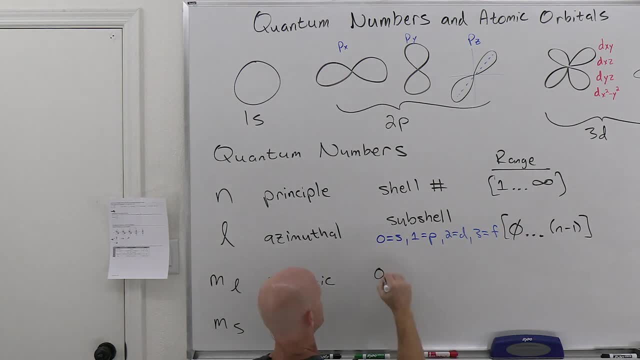 you it's going to actually identify a specific orbital. But oftentimes we say that it tells you the orientation in space, But it's going to specify an orbital, So it gives us a specific orbital And so these mean the same thing technically, Like if you look at the three different P. 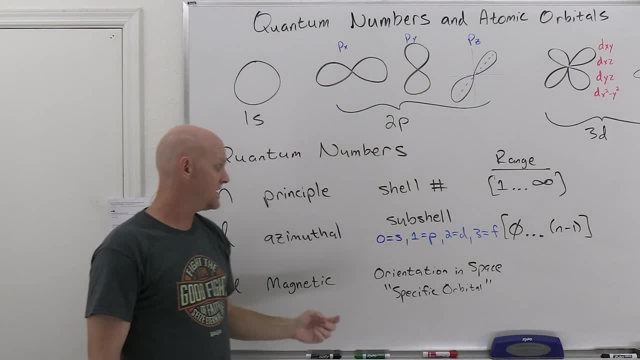 orbitals: one's on the x-axis, one's on the y-axis, one's on the z-axis. So when we say that the magnetic quantum number M sub L here specifies the orientation of the orbital, orientation in space, it's going to tell you if a P orbital is on the x-axis, on the y-axis. 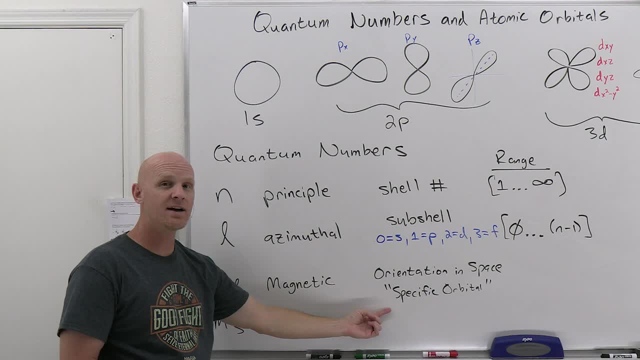 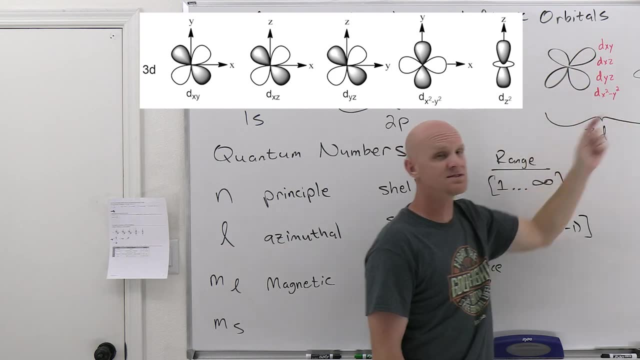 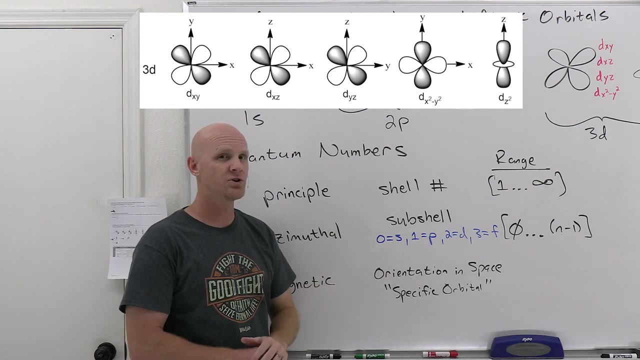 or on the z-axis. In that way, it's specifying an individual orbital in that subshell. Same thing with the D orbitals. They differ in their orientations in space And so when M sub L specifies an orientation in space, it's actually specifying an orbital in whatever subshell you're. 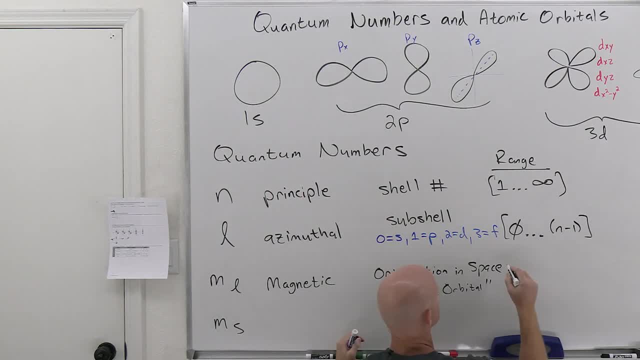 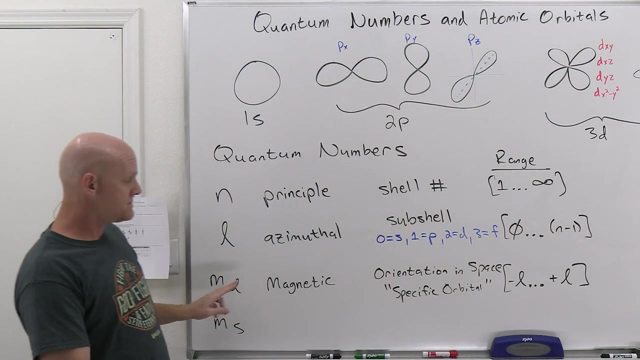 in. And it turns out, if we take a look at the range of values here, it goes from a minimum of L as an integer and all the integer values in between, up to positive L. And so, just like L is bounded by what value of N, you have, well, M sub L is going to be bounded by what value of L. 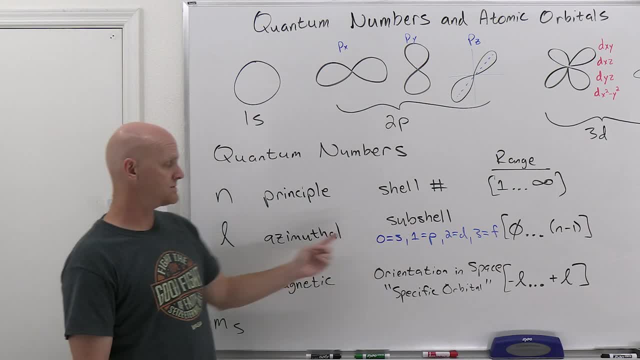 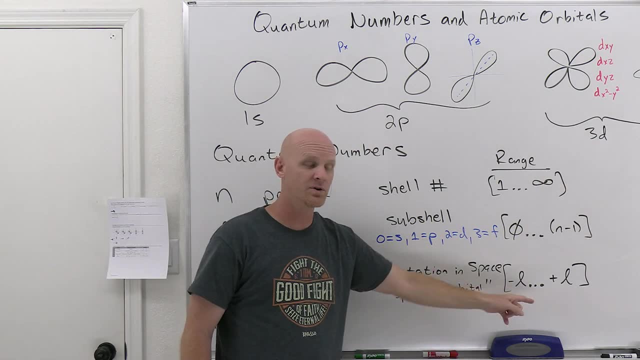 you have. So, if you have, L equals zero. L equaling zero means you're in an S subshell, And in an S subshell there's just one orbital, And so you only have to specify one orbital, And then, going from negative zero to positive zero, there's only zero. And there's only zero because you. 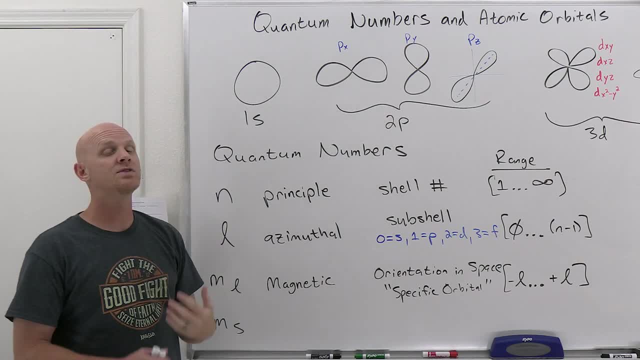 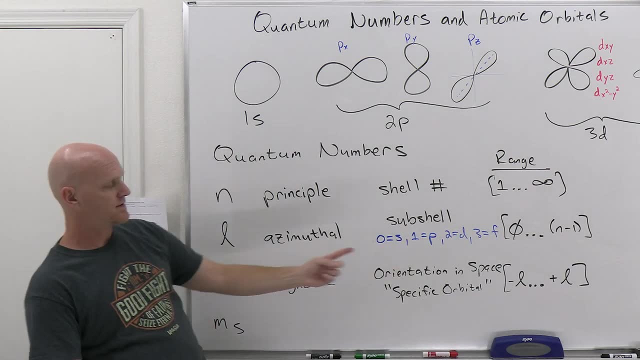 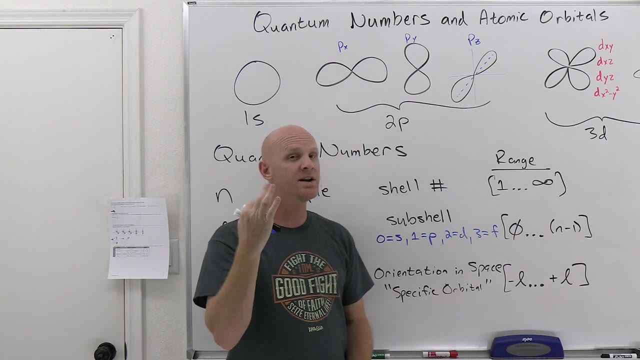 only need to specify one orbital for an S subshell. Now, if we've got a P subshell, in a P subshell, L equals one And M sub L could therefore go from negative one up to positive one. That means negative one, zero and positive one: Three different values, because we have three. 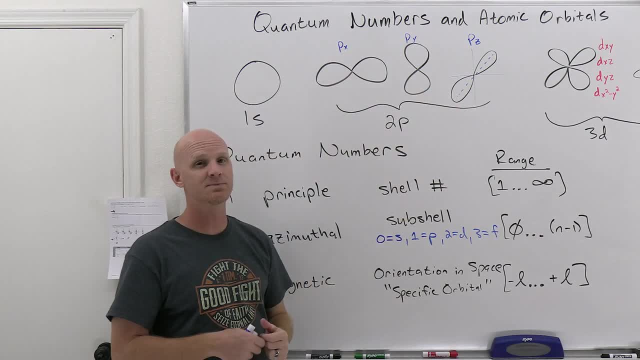 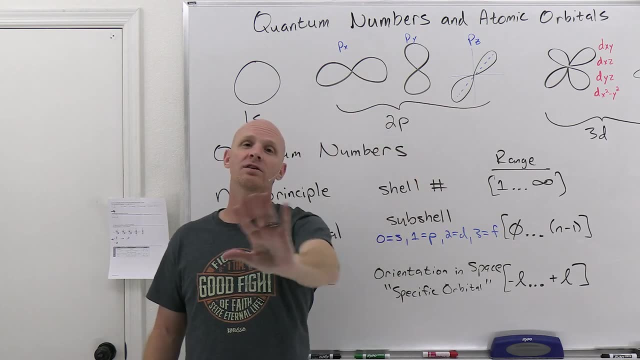 different P orbitals that we need to specify their orientation in space, And so one of these corresponds to negative one, One of them corresponds to positive one, One of them corresponds to zero, And so we have three different P orbitals that we need to specify their orientation in space, And so 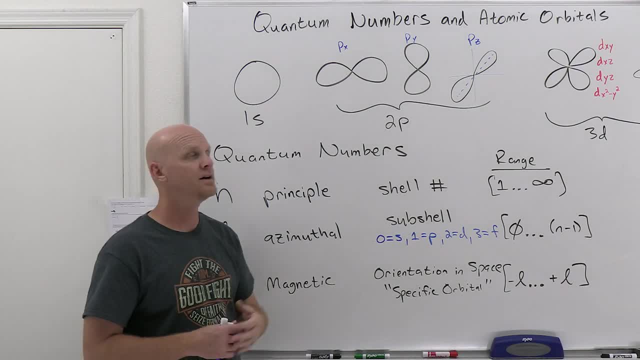 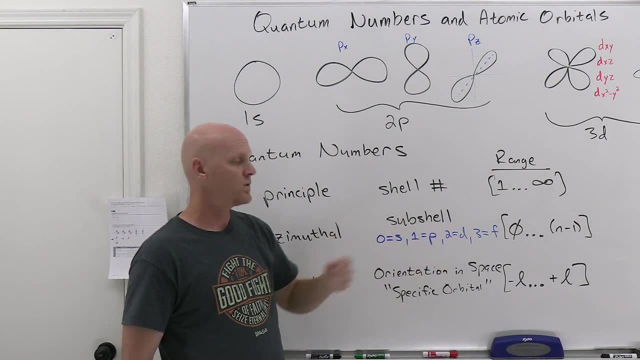 you just have to know that the three possible values would be negative, one zero and one for the P orbitals. If we go on to D orbitals, for a D orbital, L is equal to two, which means that M sub L could take on a range of values from negative two to positive two, which means negative. 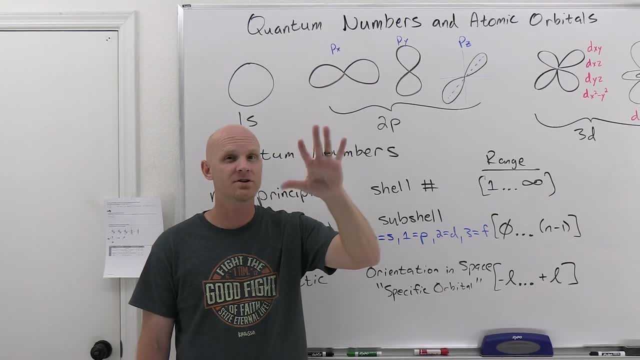 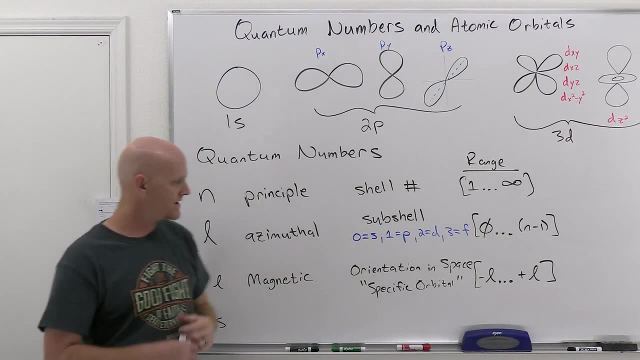 two negative, one zero positive, one positive, two, And there's five different values because there are one, two, three, four, five different D orbitals. So again, if L equals three, L equaling three means F orbital. There are seven F orbitals And that's going to allow us to get 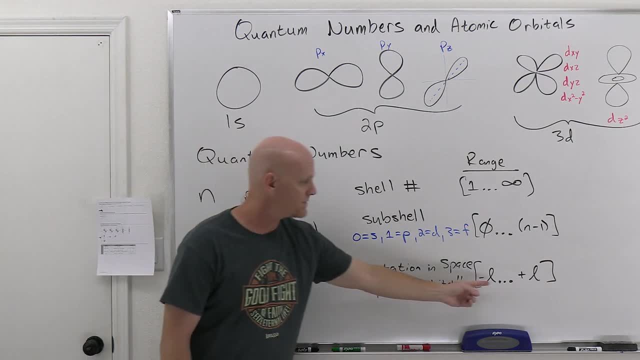 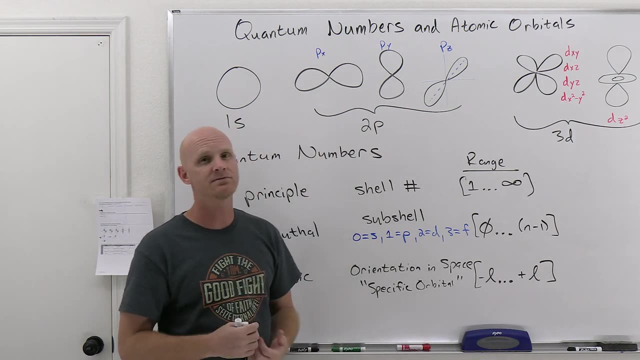 seven different values now for M sub L, So from negative three to positive three. So that means negative three, negative two, negative one, zero, positive one, positive two, positive three. Seven different values because each of those F orbitals is going to get a specific value of M. 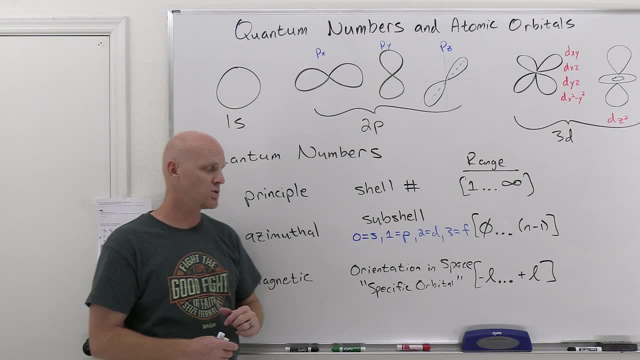 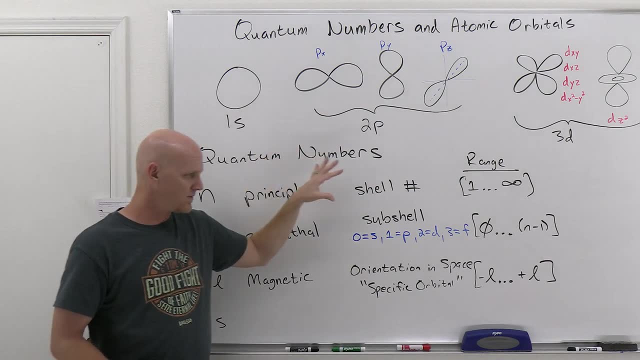 sub L because it's identifying or specifying an individual orbital. Cool, Now it turns out that these three quantum numbers, so we're kind of, you know, using them based on what they actually tell us, And they're kind of giving us an electron's. 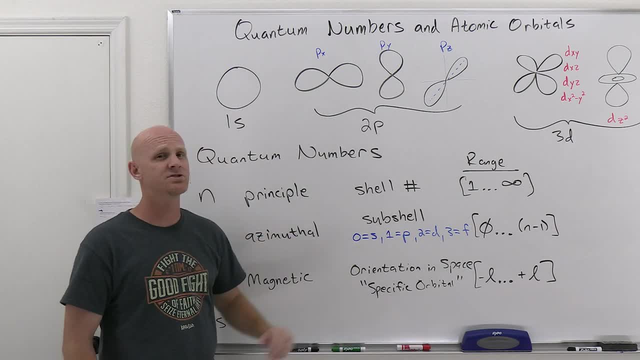 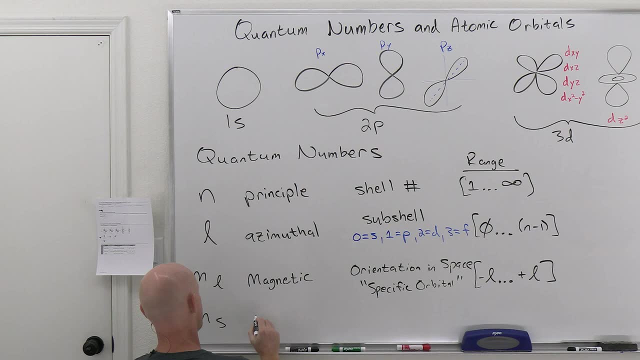 address, it turns out. But they actually come from the solutions of the Schrodinger equation. They fall right out of the Schrodinger equation. But this last one, M sub S, called the spin quantum number, does not come from the Schrodinger equation. Seen that, tested on a timer too. It's. 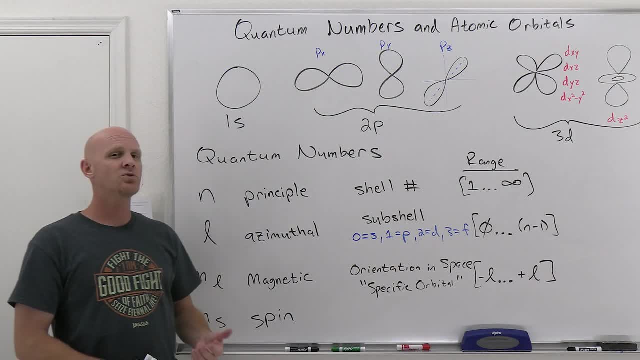 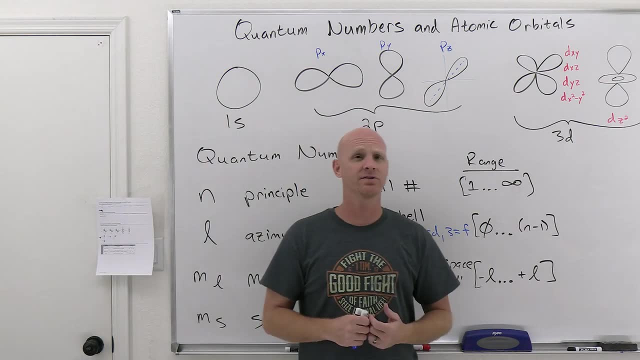 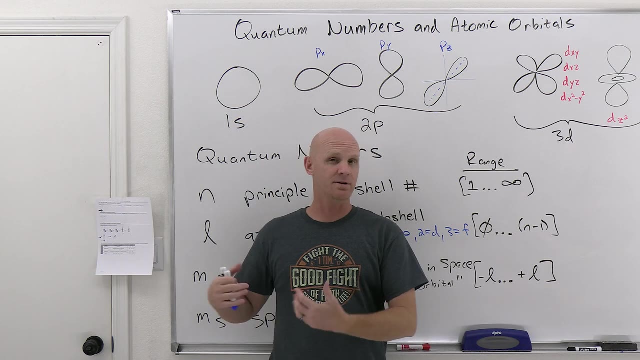 the only one that doesn't come from the Schrodinger equation. So, but it turns out that an electron has a spin associated with it, And what that spin actually is, I can't actually tell you, but it is a fundamental property of matter. So particles of matter, these individual subatomic particles, have spin. 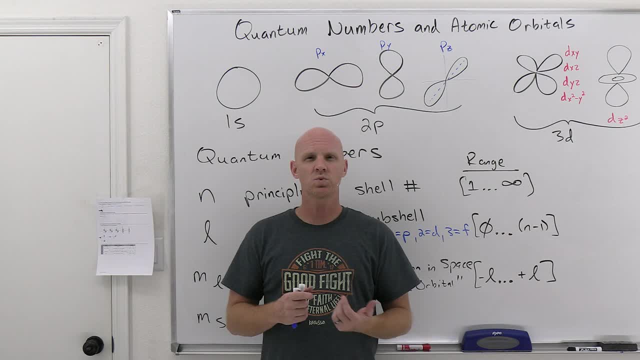 associated with them much of the time, And this spin is weird. Now it turns out that something with spin can interact with a magnetic field when it's moving, So and usually we attribute that to charged particles and things of this sort in a weird way. And the idea is that if an electron 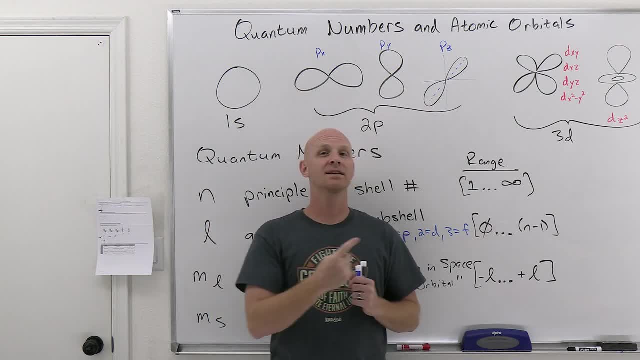 was rotating around the nucleus in one direction, it would have a magnetic field associated with it, And if it was going around the nucleus in the opposite direction, it would actually have a magnetic field associated with it in the opposite direction. Well, it turns out that these don't even have to be rotating around the 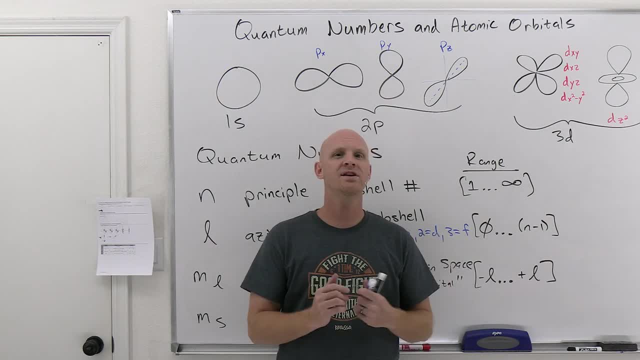 nucleus and they don't really go around in nice circular orbits anyways. And even when they're not rotating around a nucleus, they still interact with a magnetic field and have a characteristic magnetic field associated with them that allows them to interact with the magnetic field. And so it turns out it's not that they're spinning around the nucleus in any way. shape: 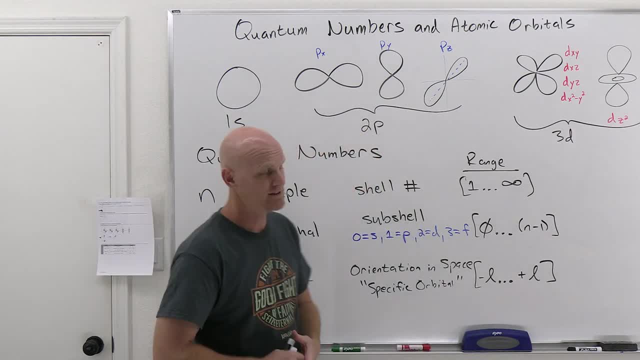 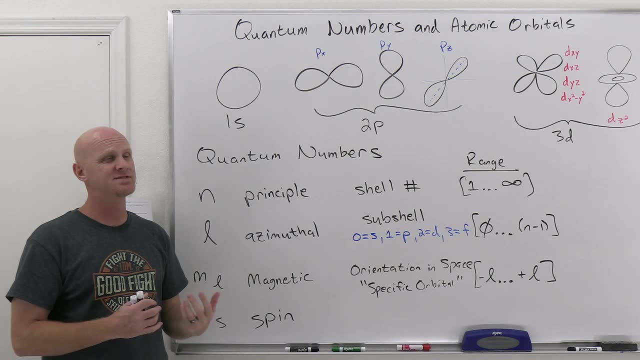 or form, It's just some fundamental property that they have. So we call it spin and based on the idea that maybe it's revolving around the nucleus, spinning around the nucleus. but it turns out that it has nothing to do with that. It's just a fundamental, inherent property of electrons. 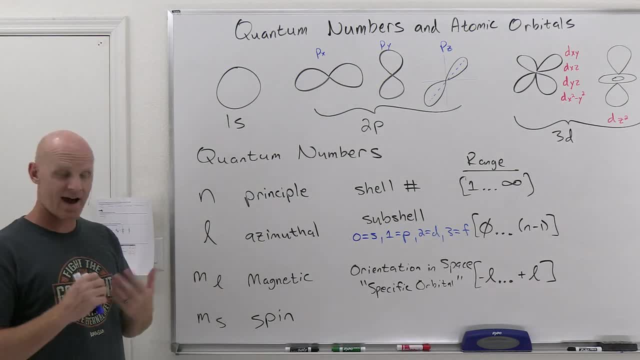 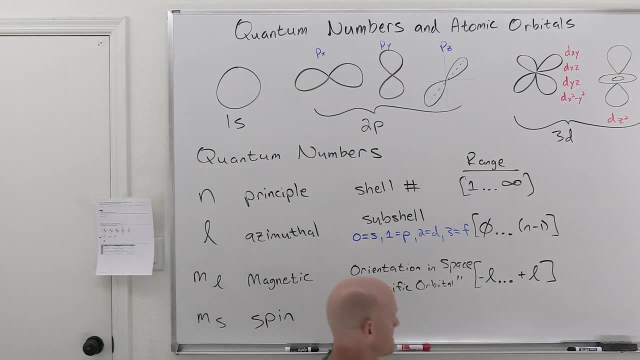 And it's not just electrons. Most particles have a spin associated with them. Okay, it turns out that this spin is actually what we're going to represent here. It takes on two possible values. It is either plus one half or minus one half. 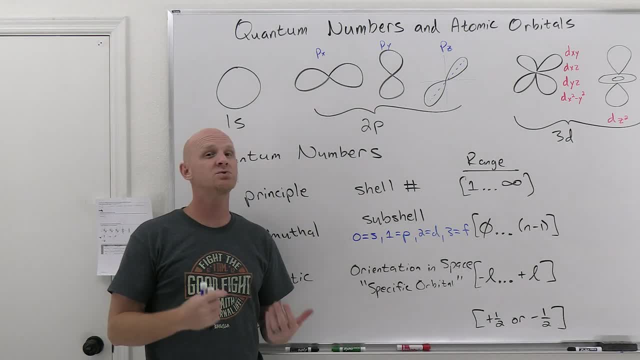 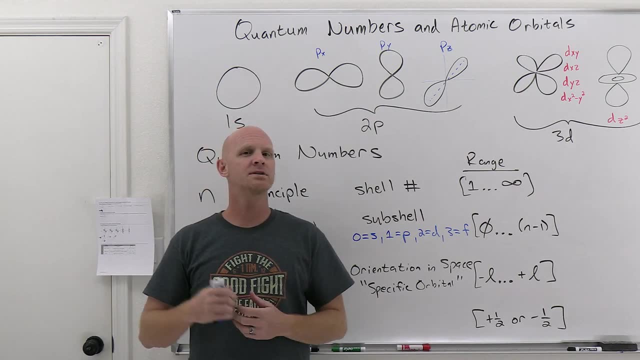 this range of values. there's just two values possible, And so it turns out there's only two types of spin. So- and you can kind of think of this- there's only two types of charge in the universe, and we identified them as positive and negative charges. Now notice, that's just what. 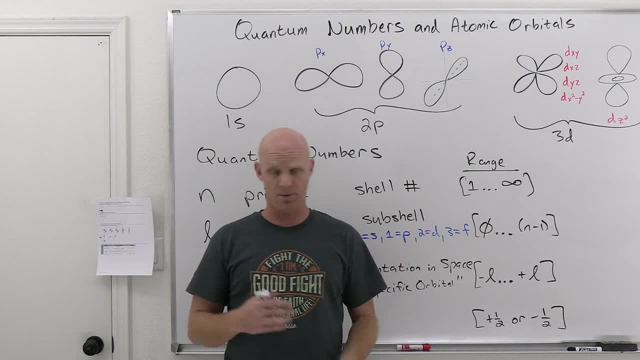 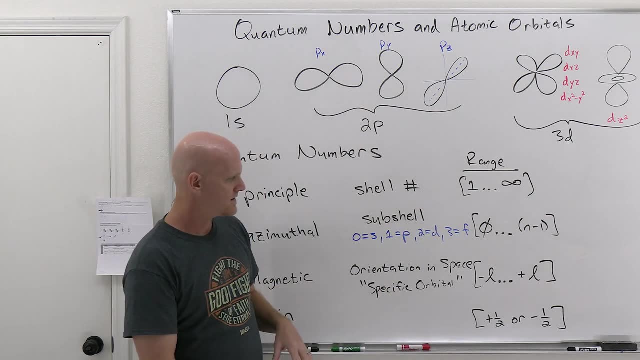 somebody called them. We could have called them left charges and right charges, or up charges and down charges, or blue charges and green charges, or we could have called them anything and just known they were opposites. So well, here we've got these opposite spins, but it turns out they. 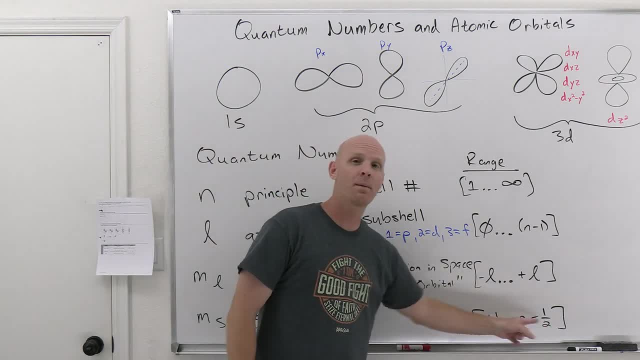 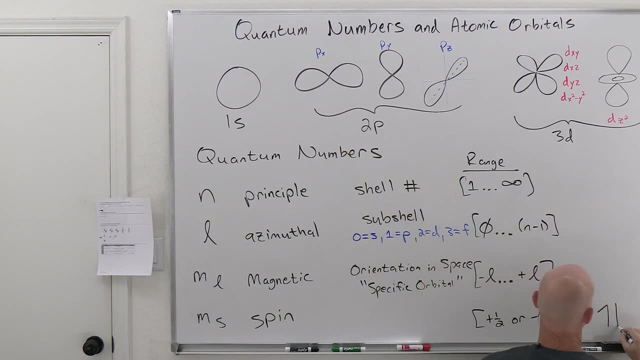 have actual numerical values associated with them that are indeed opposites. So plus one half and minus one half, And we're going to find out that we're going to represent electrons here in a little bit with arrows like so, And we're going to have one arrow point up and one arrow point down. 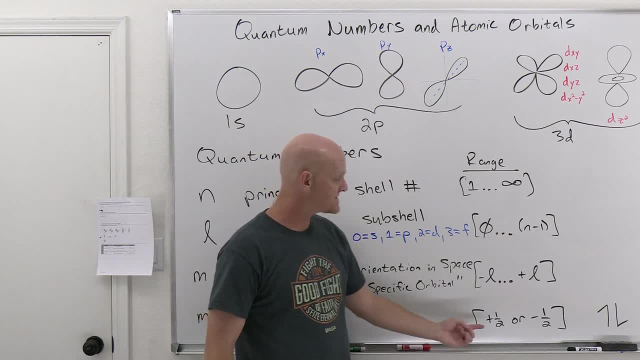 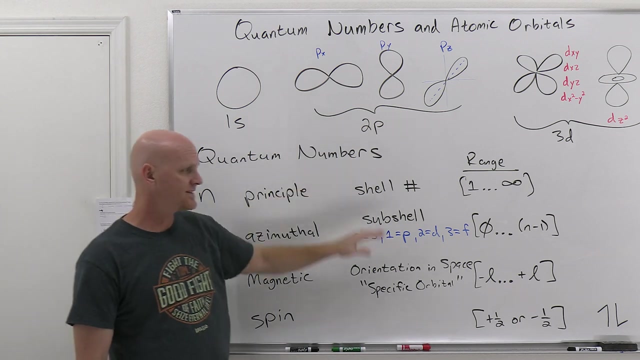 And these arrows represent electrons and we represent the opposite spin quantum numbers for them by representing the arrows pointing in opposite directions. Now we've got these lovely four quantum numbers here And in this case we know their names, we know their symbols, we know what they tell us. And now 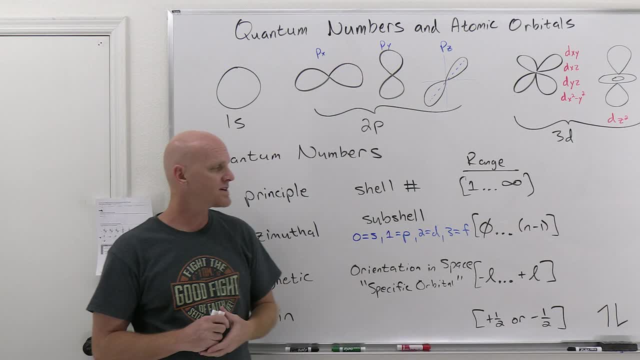 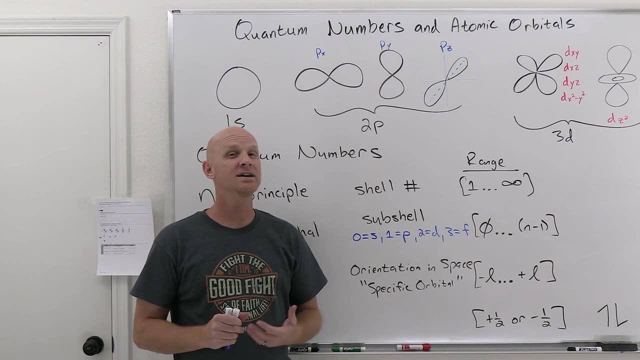 we know the range of values they can take, And there's a few different kinds of questions you might have to answer. Now, one thing: we got to give a prelude to the next lesson, and that's called the. we got to talk about what's called the Pauli exclusion principle, And it's essentially 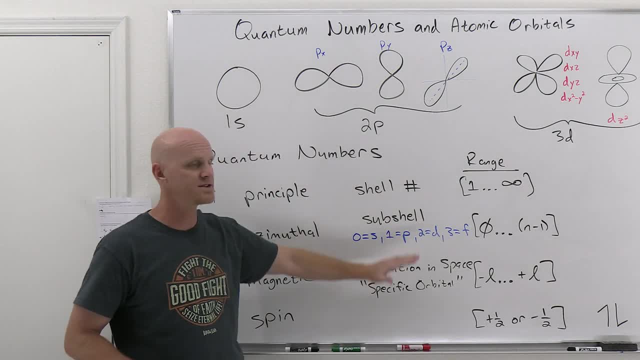 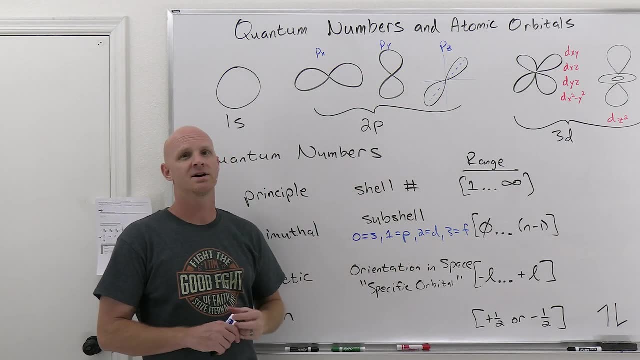 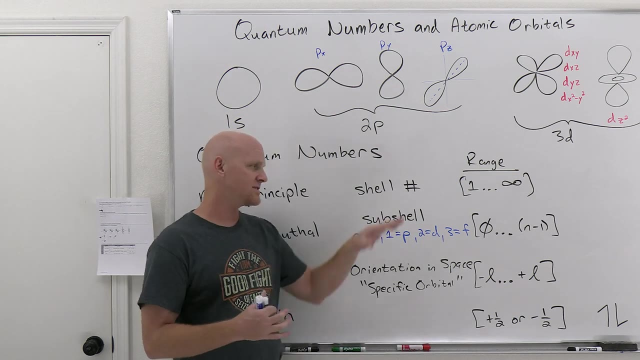 excludes any two electrons from having the same four quantum numbers. So every electron in an atom is described by some combination of four quantum numbers, and no two electrons in an atom can have exactly the same set of four quantum numbers. What that ultimately means? because, again, 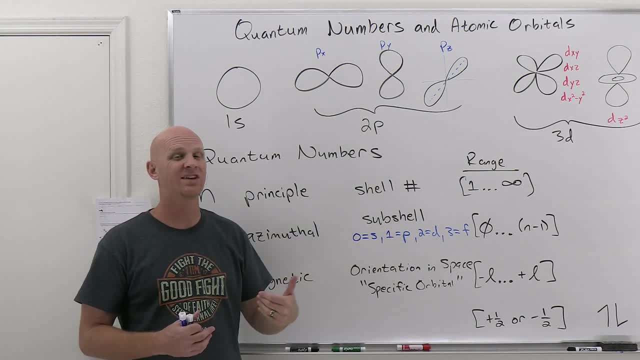 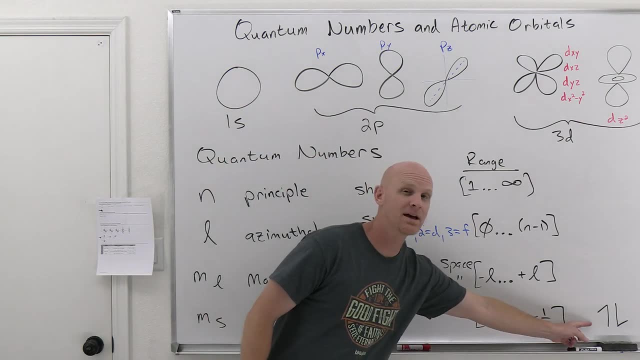 the set of four quantum numbers ultimately describes an electron's address. It means that no two electrons can live in the same orbital and have the same spin, as it turns out Now, what do I mean by these being like an electron's address? Well, think about. 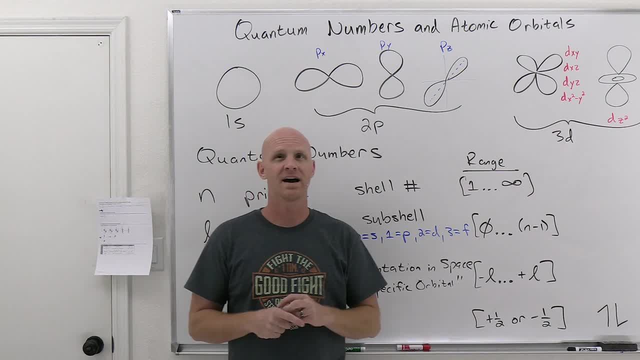 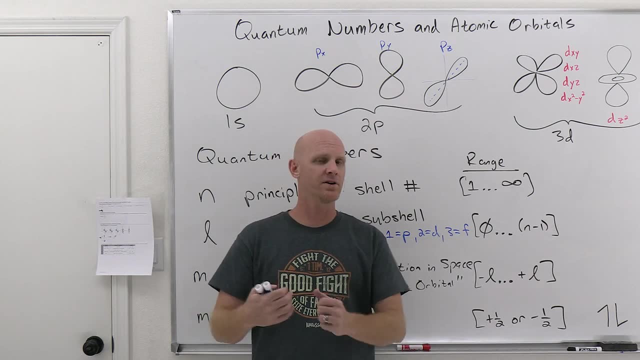 think about this. Let's say, I gave you my address and I said that I live in state number 48. And so I didn't tell you what state I lived in. I just assigned a number value to my state. Well, if you've heard it- heard me say it in other videos- I live in Arizona, And the reason I call 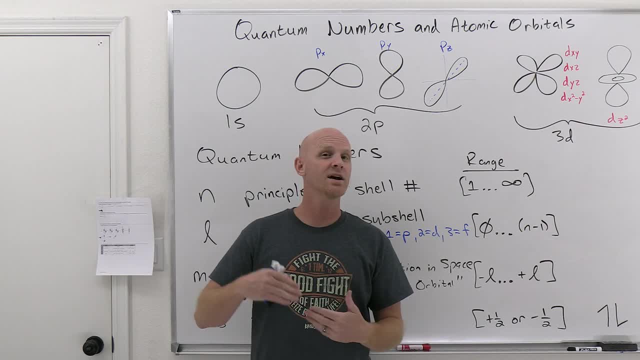 it state 48, that was a code, because Arizona was the 48th state to be made a state in the union, if you will. So that's where that code comes from. And then maybe I tell you: Hey, I live in. 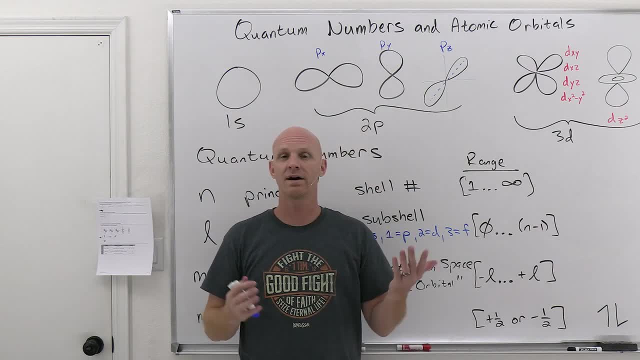 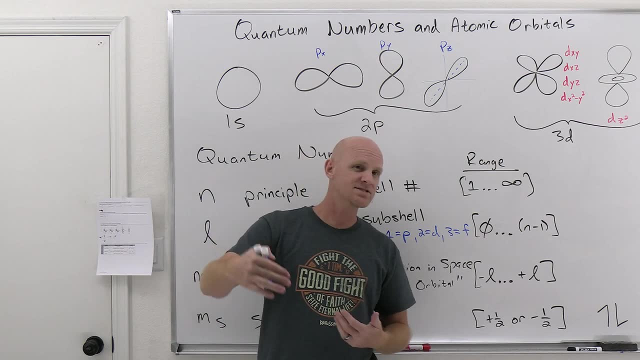 city number seven. So, and again, you might start doing some research and find out: you know what was the seventh city in Arizona, And I have no idea if this is correct, but I live in Tempe, So we'd be like, Oh, the seventh city in Arizona was you know. 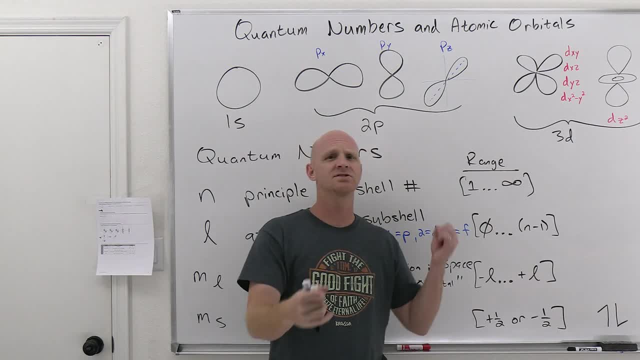 Tempe, And I'm just giving you a code, And so I'm like I live in state 48.. I live in city number seven And so, and then I might tell you I live in street 104.. And then we might do some research. 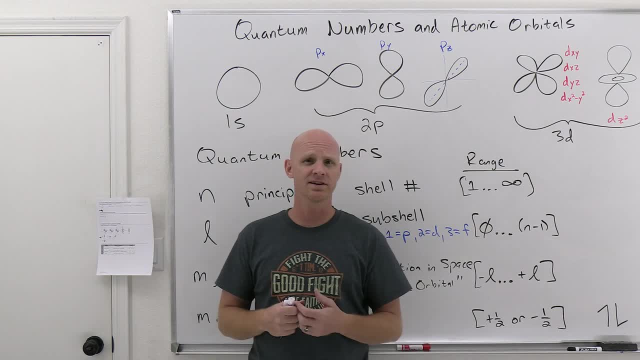 and find out what was the 104th street to be paved in the city of Tempe, or something like that, And then I might finally give you a house number. And so, instead of giving you my address in normal terms like house number, street, city state, I'm giving you numerical values as a code for this. 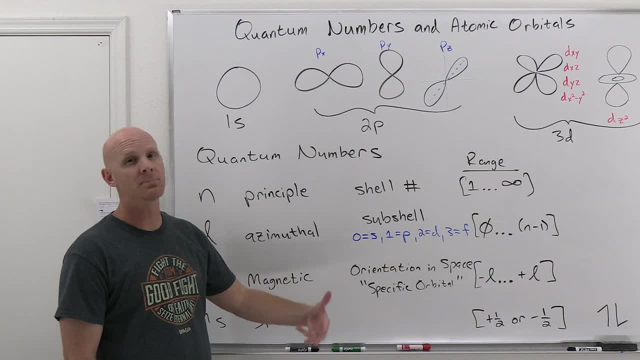 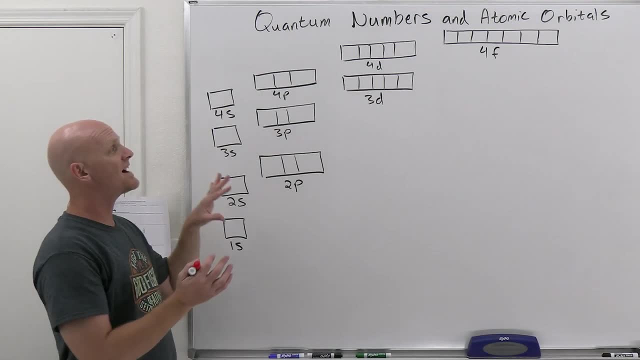 Well, we're doing the same thing here. When I give you a set of four quantum numbers, it's a code for where an electron lives, And we'll take a look at how this works here. All right, So here's a common diagram we use to represent the energy location for the different. 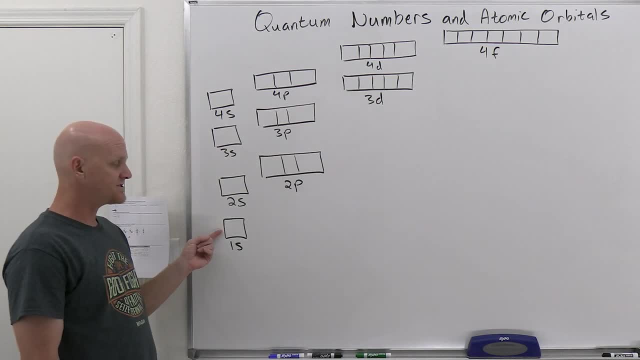 subshells and orbitals in an atom and the lowest energy orbitals of one S. So this box represents the orbital and then we're going to draw arrows inside these boxes to represent the electron. So we might put an electron like here And then when the next one turns out we'd have to draw. 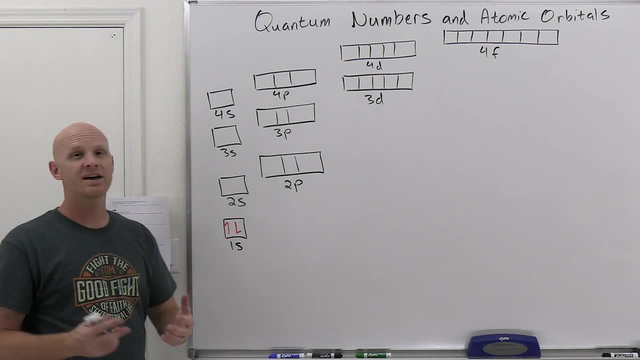 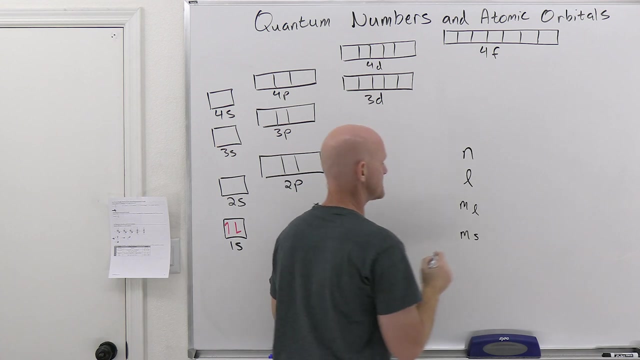 would be spin down. So it turns out one spin up, one spin down, And again that corresponds to the values of the spin quantum number. as we'll see, And based on where an electron is found somewhere in this diagram, we can assign values to N, L, M sub L and M sub S, And what you'll find is that 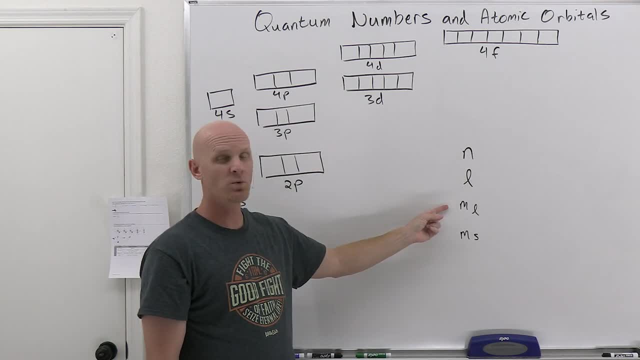 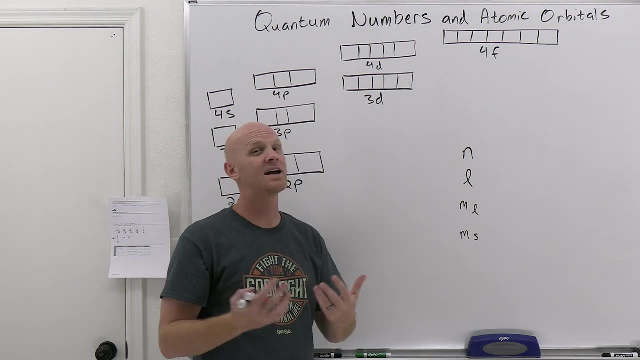 most of the time you can assign a specific value to N and L, but you might have a range of values that are possible for M sub L and you might not be able to specify which it is. And then M sub S. you're probably just going to know it's either plus one half or minus one half, and good chance. 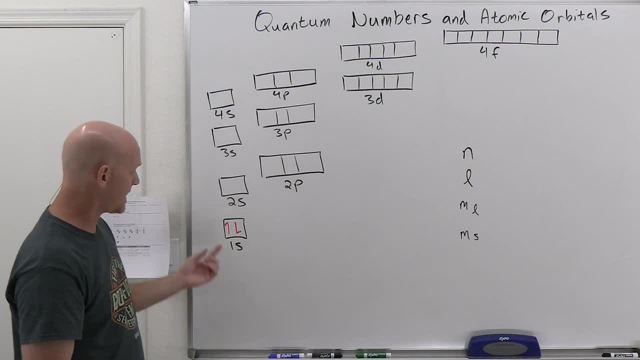 you might not know which is which. All right, So let's say we talk about one of these electrons, It doesn't matter which one, Let's just erase one of them and say we're talking about one of those one S electrons, So that electron, and we might say what is its set of quantum numbers? Well, 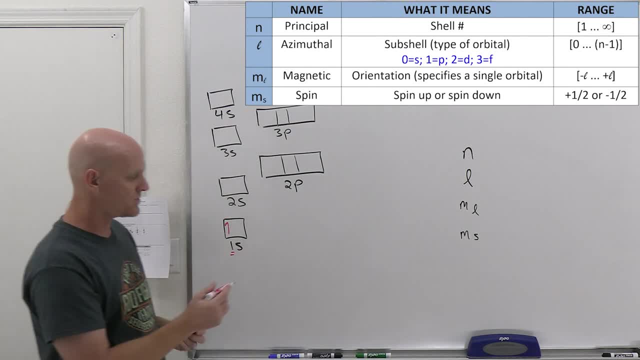 it is in shell number one here, and that one is the principal quantum number, And so here N would equal one. So, and then L, since we're in an S sub shell, you remember L tells you the code: L equals zero means S, L equals one means P, L equals two means D, L equals. 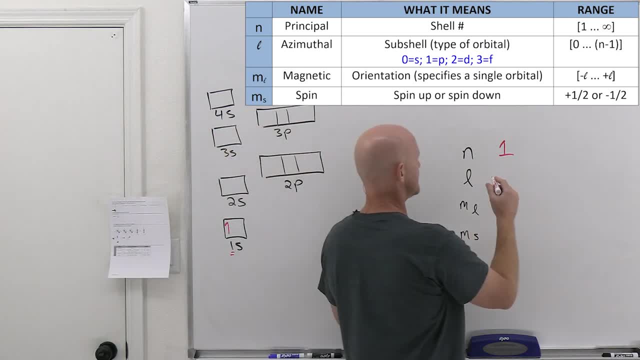 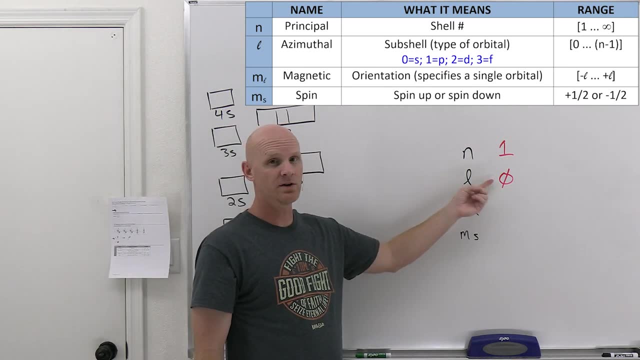 three means F. So in this case, because it's an S sub shell, that that electron is in L is going zero. And then you recall that M sub L takes on values from negative L to positive L. So in this case, from negative zero to positive zero means the only possible value is zero. Cool. And then 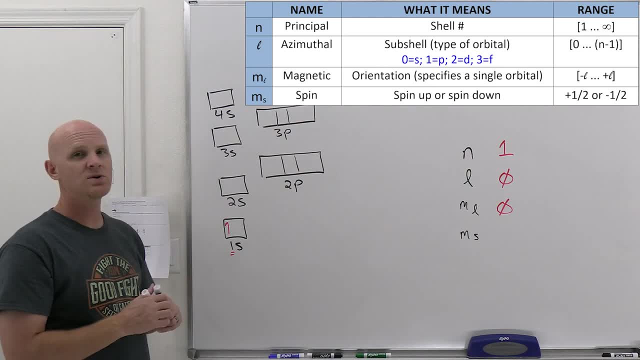 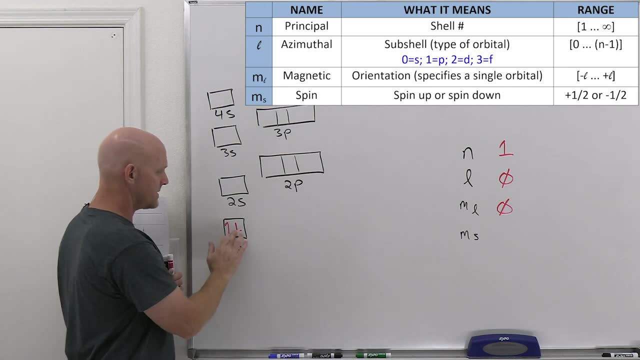 finally, M sub S. Well, again, we said that when you have two electrons in the same orbital, we would draw them as one spin up, one spin down. So, and in this case, when you only draw one of them, though, and it doesn't matter if it's spin up or spin down, we actually don't specify that. 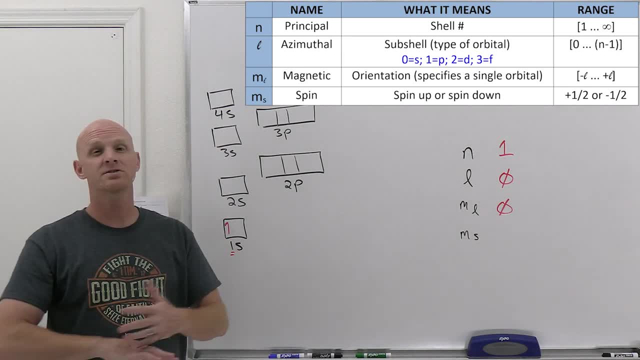 you know, spin up means plus one half And spin down means minus one half. There's no specificity there at all. We just know we have one of them. This is either the plus one half spin or the minus one half spin, We don't know which. 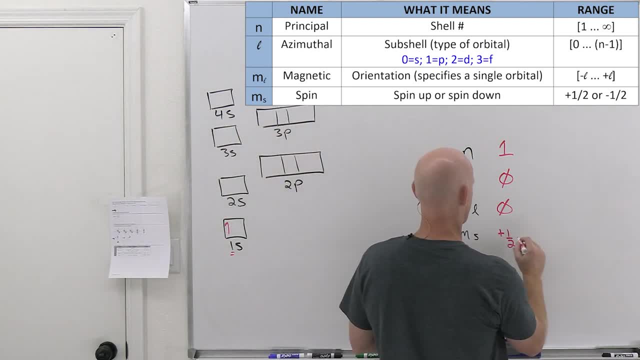 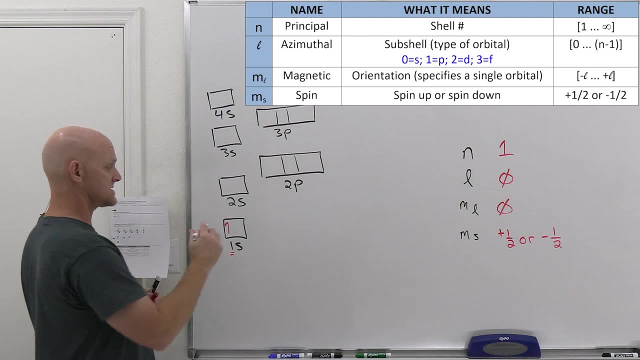 And so all we can say here is that it's either plus one half or minus one half, And we can't get any more specific to that. Now, what I could tell you is this: If I drew both electrons in in this particular orbital and if I told you the one on the left is the minus one half electron, 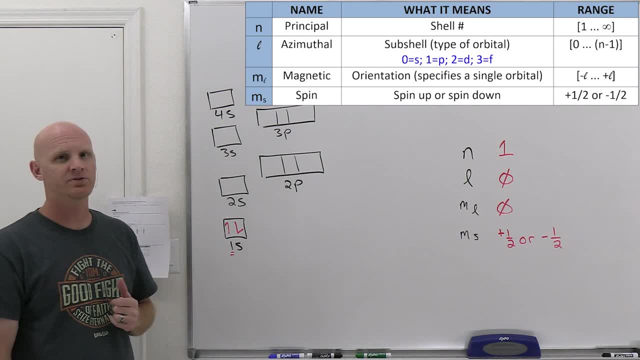 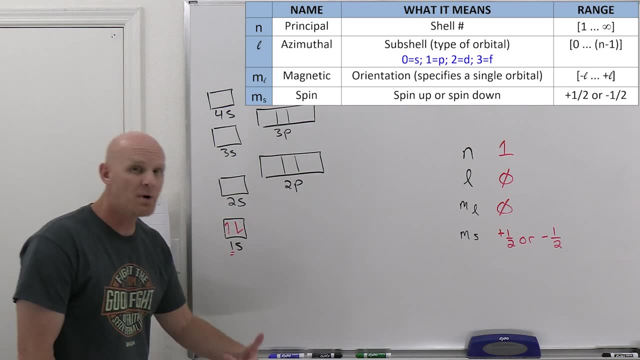 well then you'd know that the one on the right would have to be the plus one half electron, And the key is they have to have opposite spins, because if they had the same spin, if they were both plus one half or both minus one half, well they're both in shell number. 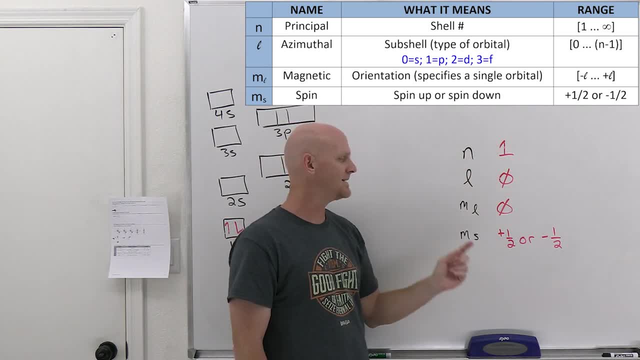 one. They're both in the S orbital. They're both in the same S orbital And if they had the same spin, then they would have the same four quantum numbers. And again, the Pauli exclusion principle tells us that that is not possible. And it's not possible because Pauli said so. Pauli was just 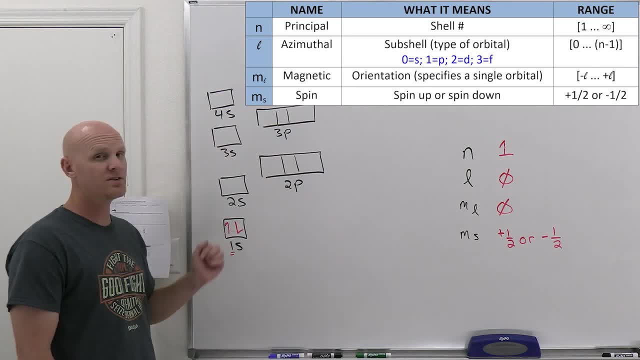 describing nature. It just turns out that nature doesn't put two electrons in the same orbital with the same spin. It's just the way it works. And so you know we can't say: that's the way it works, Cool, So that was that electron. So let's say we put an electron somewhere else in this lovely atom. 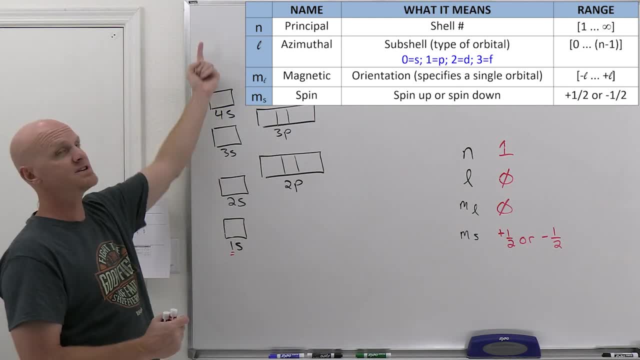 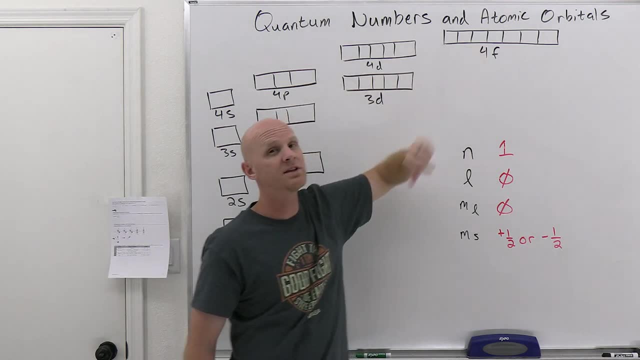 And so a couple of things you should realize about the orbitals here is that we're going increasing energy as we go up. So notice shell one is lower than shell two, Shell two is lower than shell three And shell three is lower than shell number four of electrons. But also note that 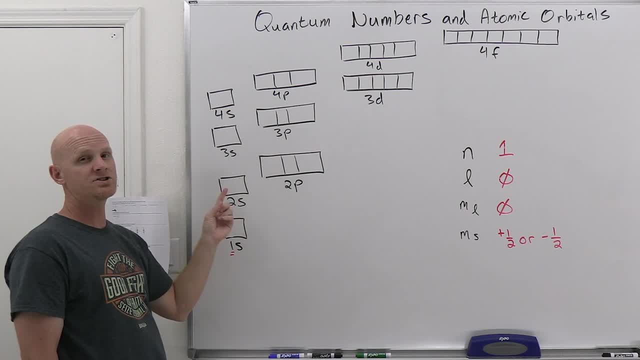 you know, when you get to the higher shells, you got like S's and P's: The P's are higher in energy than the S, The D's are higher than energy than the P, which are higher energy than the S. And 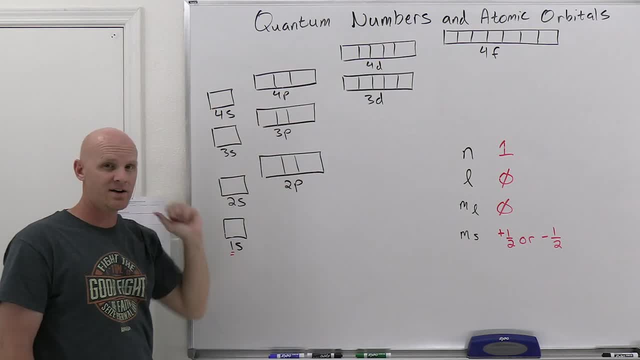 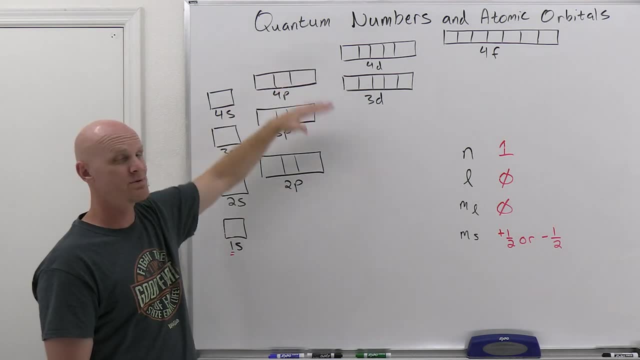 then F are higher energy than D, are higher energy than the S, And then P's are higher energy than the S. So for any system that only has one electron, it turns out that the way this is represented is not true. And the most notable atom or ion that only has one electron is hydrogen. And for something? with only one electron, most notably, again, the only neutral species of hydrogen. it turns out that all the subshells and orbitals within a single shell are going to be equal, So, instead of having the P higher than S, they would all be at the same level, all the same energy, And that's only true. 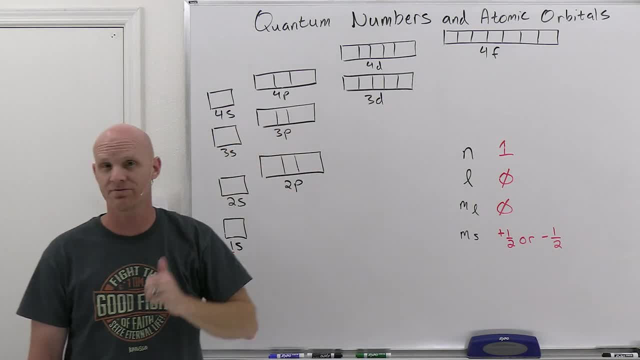 for one electron system. Same thing here: 3S, 3P, 3D For hydrogen. they're all equal energy. But for any multi-electron system they split into different energies And we'll talk about that at a much. 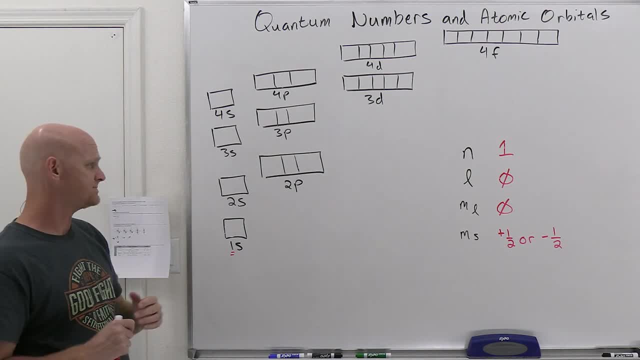 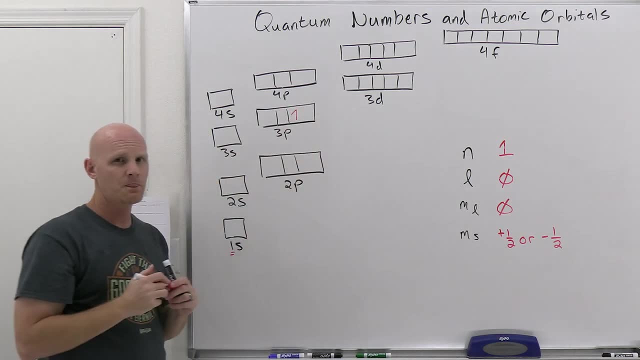 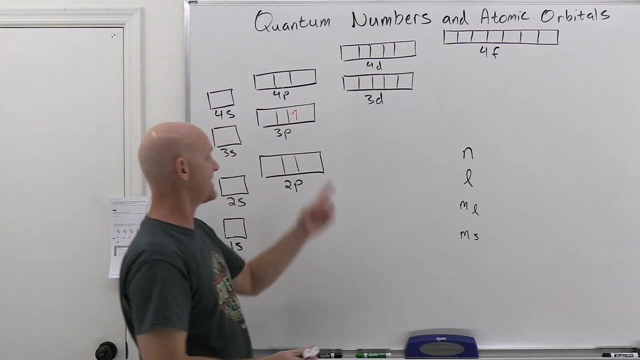 later date why that is and stuff like that. So just something you should realize. All right, so let's say we've got an electron now and let's put this electron right here, And so now the questions again are: what is the possible sets of four quantum numbers that that electron could have? 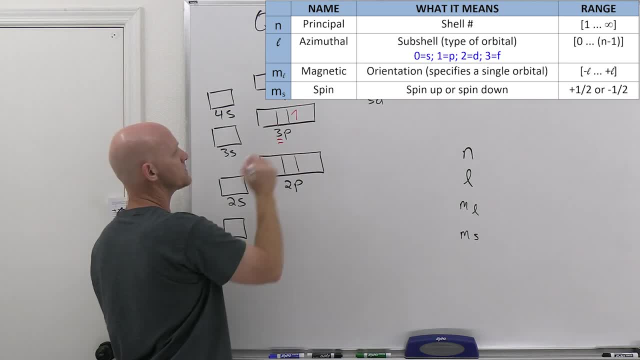 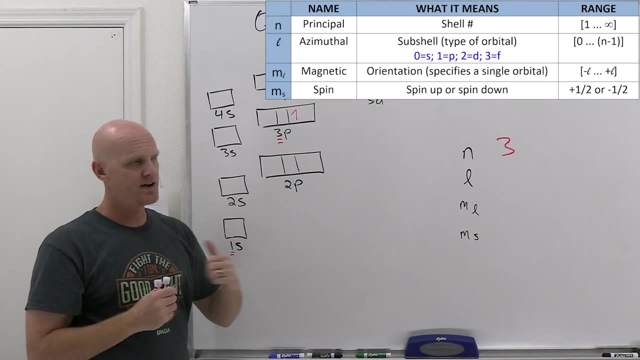 Well, let's say we've got an electron in the 3P, So that means it's in shell number 3. So n is going to equal 3. And it's in a P subshell. And again L tells you the subshell And the P subshell. 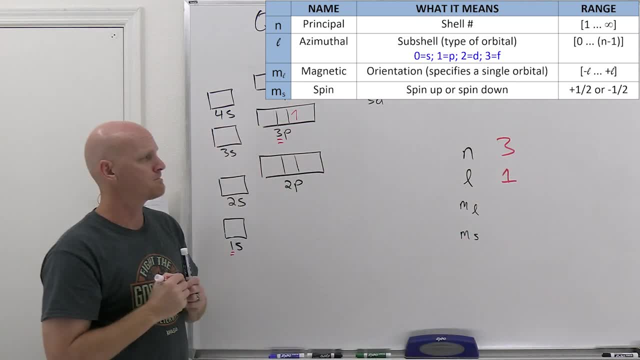 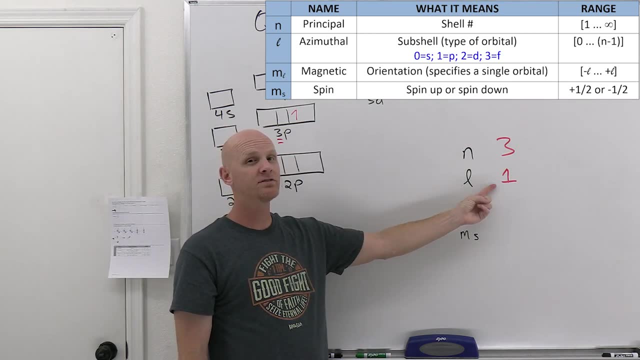 corresponds to L, equals 1.. Cool, Now here's the deal. We've got to go to M sub L, And M sub L takes on a range of values from negative L to positive L, So in this case, negative 1 to positive 1.. 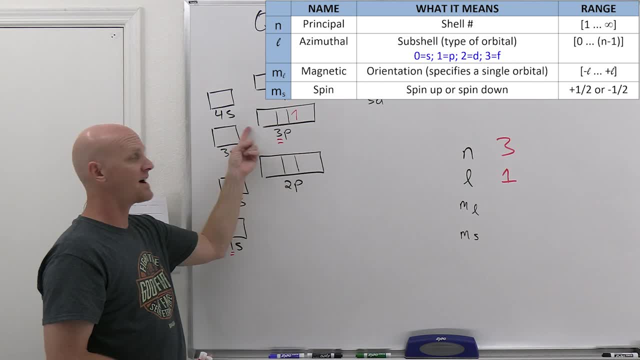 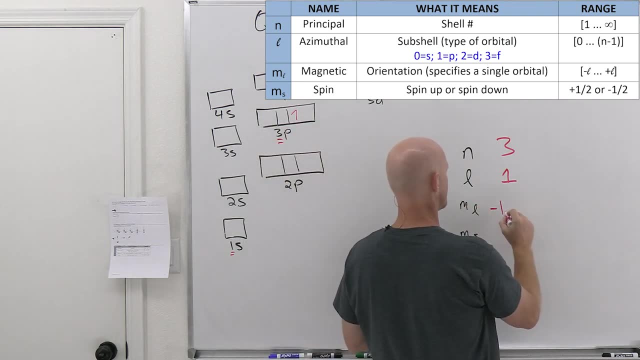 So either negative 1, 0, or positive 1.. And on a diagram like this we don't specify It could be any of those three, And so we can't actually get it specific here. We can only say that it's either negative 1, 0, or plus 1.. It's one of those three, It can't be. 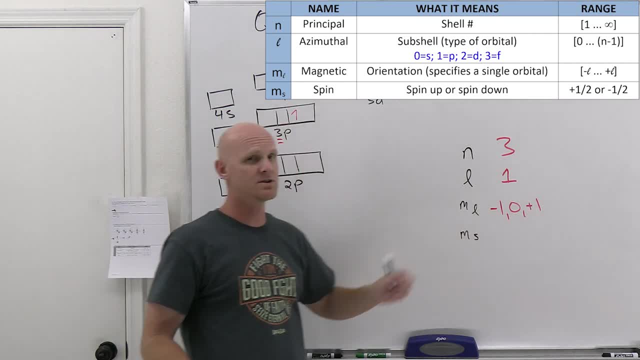 negative 2.. It can't be positive 3. But it's got to be one of these three specific values, But can't get any more specific than that. And then finally, M sub S same thing as before, It's either plus. 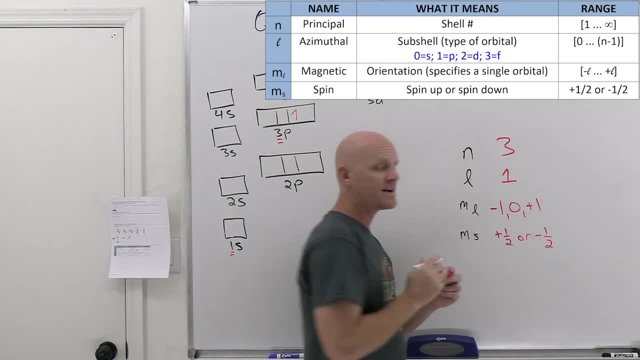 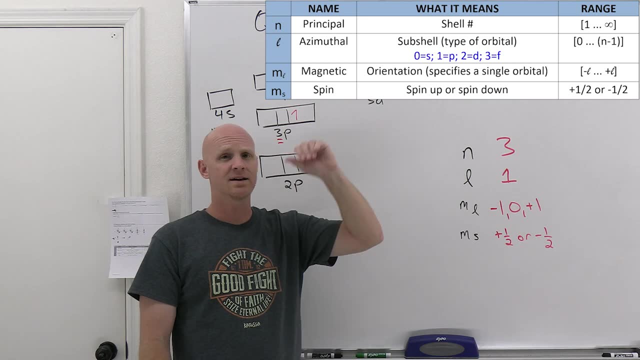 1 half, or it's minus 1 half, And we can't get any more specific than that either, And so you might get a question on the test that says you know multiple choice. let's say: And which of the following is a possible set of quantum? 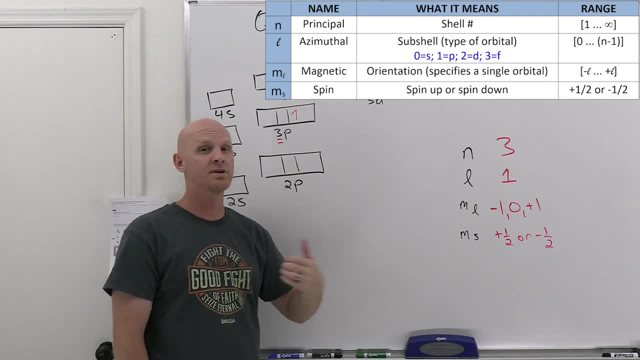 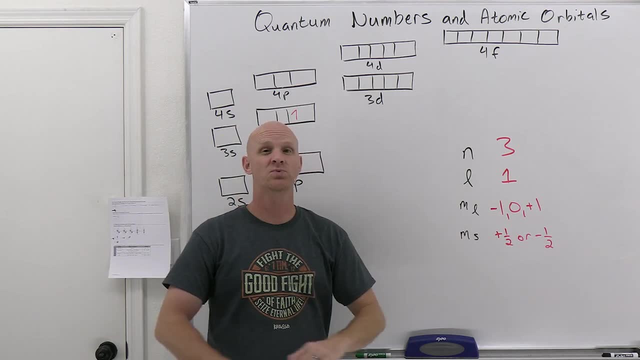 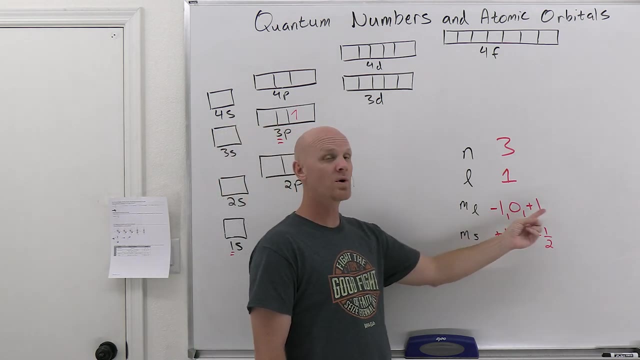 numbers for that electron right there Or for an electron in a 3P orbital. Well, any answer that doesn't have N equals 3 is wrong. Any answer that doesn't have L equals 1 is wrong. But notice for M sub L. there are three possible correct answers here: Either negative 1, 0, or positive 1.. And 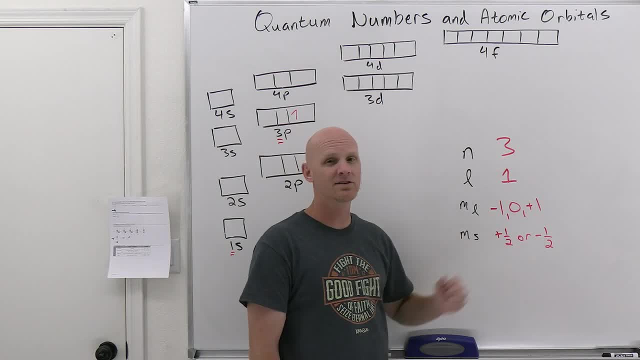 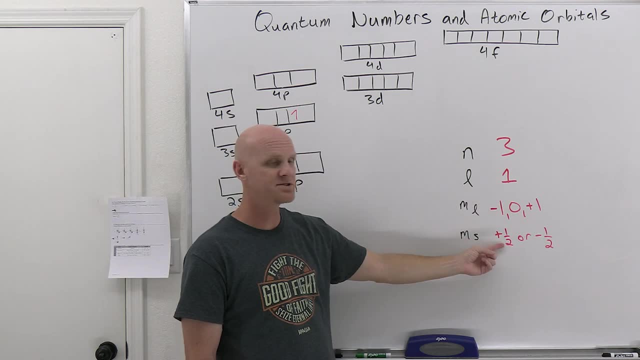 then for M sub S, there are two possible correct answers, plus 1 half and minus 1 half, And you've got to find the combination of four That are all within this range. So with three different options here and two different options, 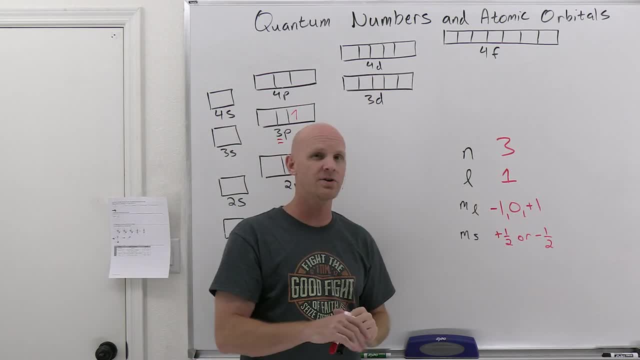 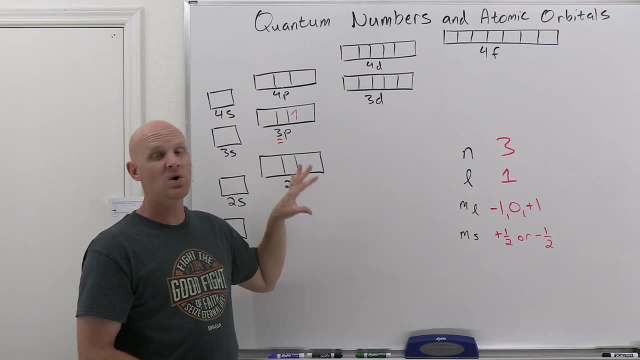 here. there would actually be six possible correct answers that could include on your answer sheet. Obviously, they're only going to include one of those options as a correct answer. Cool, The other way you could see quantum numbers showing up is they might just start giving you. 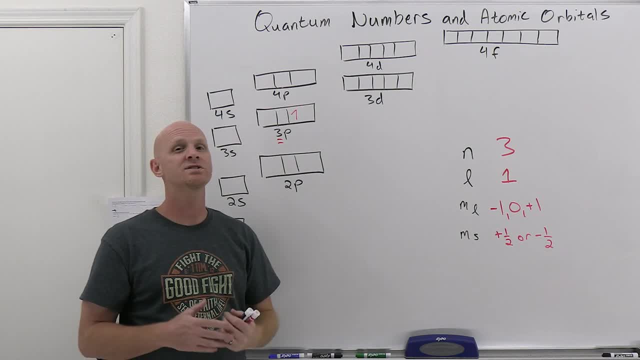 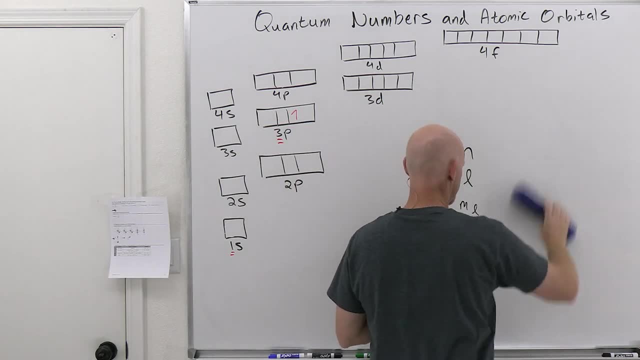 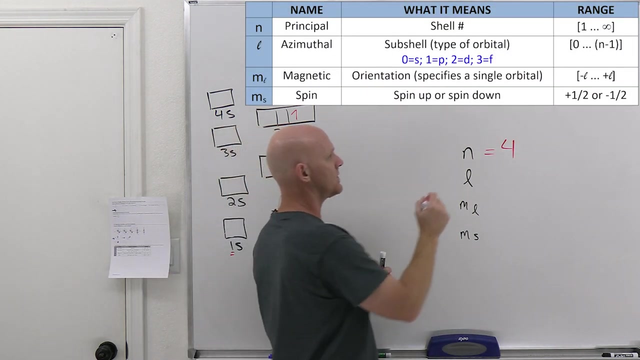 different combinations of quantum numbers and asking which of the following is even possible. So which of the following is a possible set of quantum numbers? So let's say, we start messing with this a little bit- you that n equals 4.. Is that possible? Yes, But what if I told you it was n equals negative 4?? 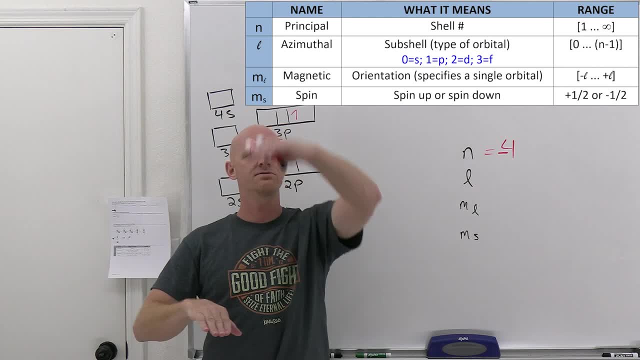 Well again, n only takes on a range of values from 1 at the lowest up to infinity. It can't be a negative number. So whatever else we fill in for l, m sub l and m sub s, this would not be a. 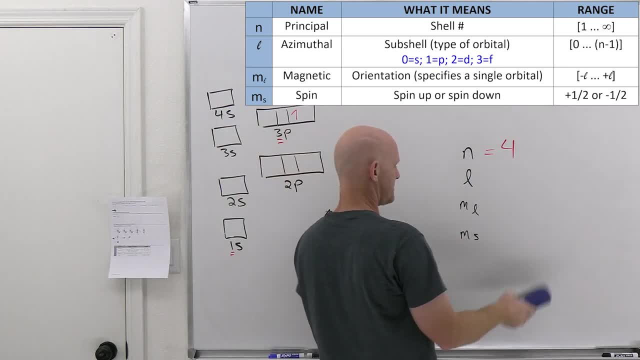 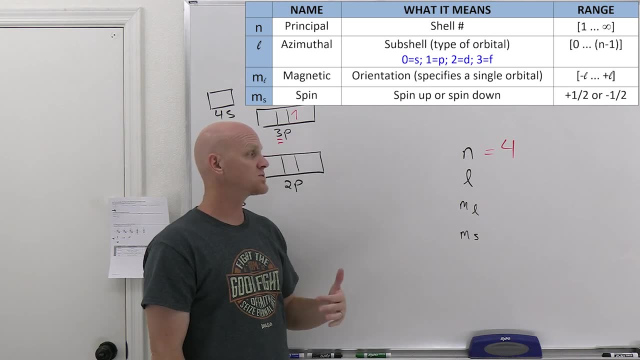 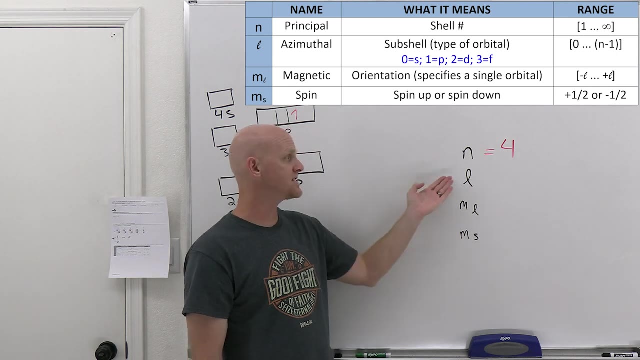 possible set of quantum numbers. But as long as I just said, n equals plain old 4, positive 4,. okay, so far, so good. Now, what values could l have here? Well, in this case, you remember that l takes on a range of values from 0 at the minimum, to a maximum of n minus 1, in this case, 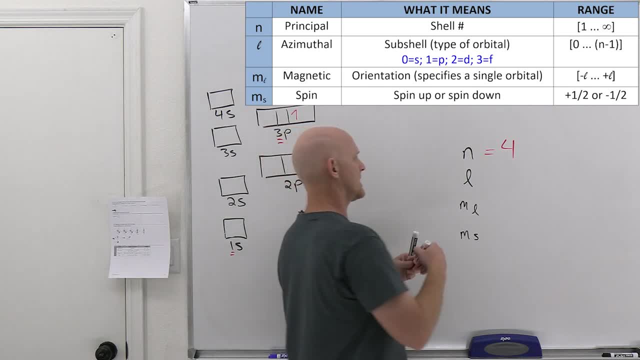 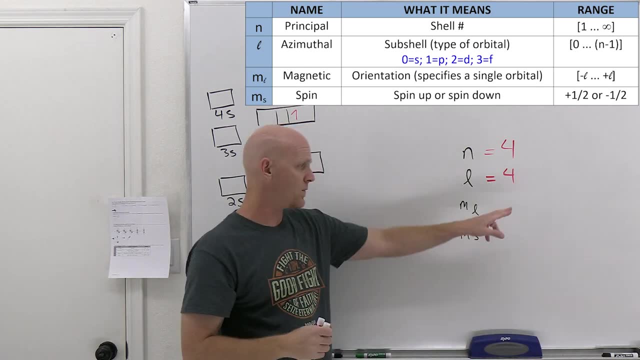 to a maximum of 3.. And so, in this case, if I put, let's not, let's just say 4 again, well, then again, no matter what I fill in for m sub l and m sub s, you'd know that this is not a possible. 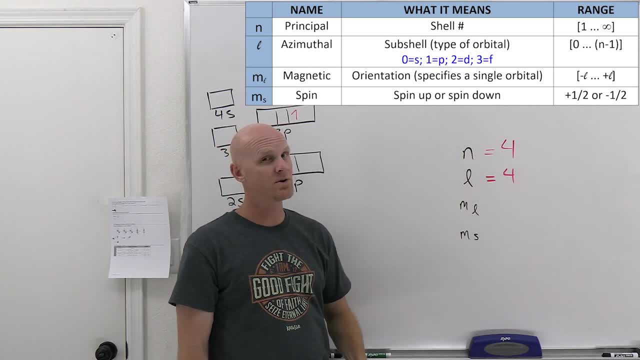 set of quantum numbers, because with n equals 4, l could be 0,, 1,, 2, or 3, but it couldn't be anything greater than that, So that wouldn't be possible anymore. Okay, so we're going to go ahead and do that again. So we're going to go ahead and do that again. 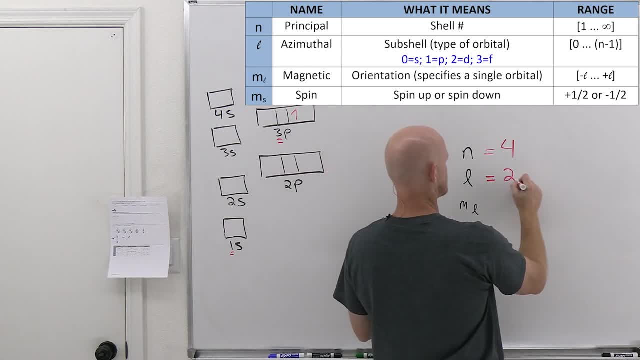 Okay, so we're going to go ahead and do that again. So we're going to go ahead and do that again. Let's say I put one of the possible numbers. let's say I put l equals 2.. And again it could have been 0,, 1,, 2, or 3,, but no higher than 3.. So this is possible though. 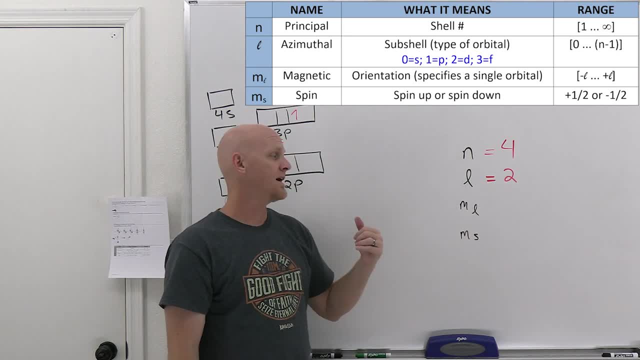 Okay, so let me move on to m sub l, And in this case m sub l depends on the value of l, in the same way that l depended on the value of n, And for m sub l it takes on a range of values from: 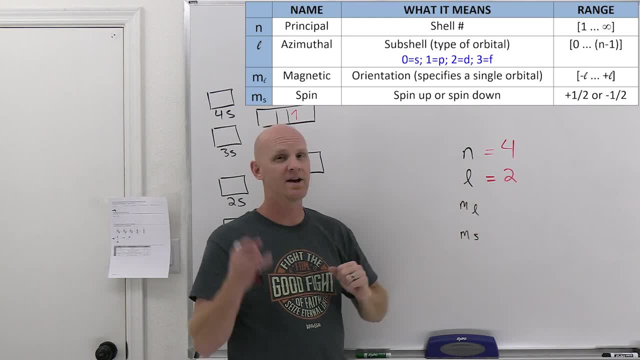 negative l to positive l, those integer values in between. So negative 2, negative 1, 0, plus 1, plus 2.. So if here again I put minus 4,, well, that's outside the range of possible values. And again, no matter what I fill in for m sub s. 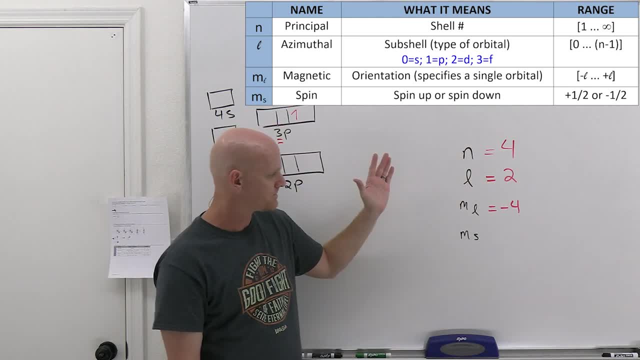 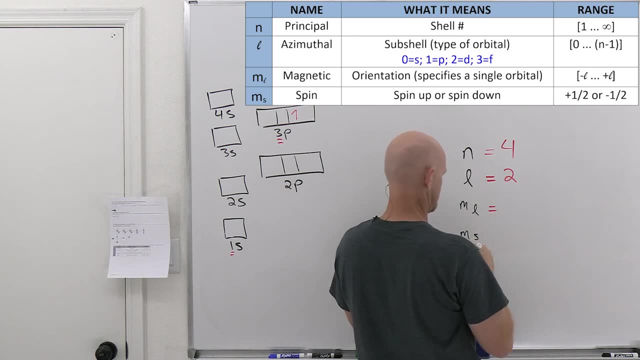 this would not be a possible set of quantum numbers for anything. So again, outside that range of negative 2 to positive 2.. But once again, if I go in and say, how about negative 1, that works. It could have been negative 2,, negative 1,, 0, plus 1,. 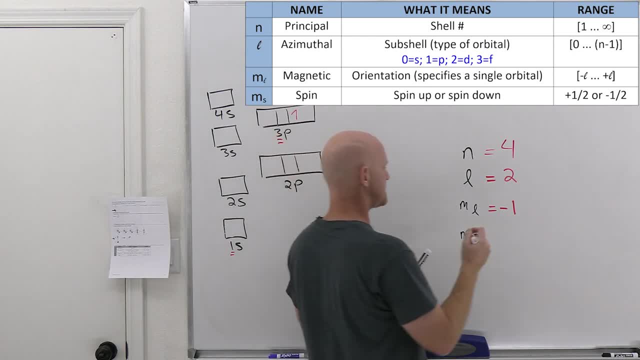 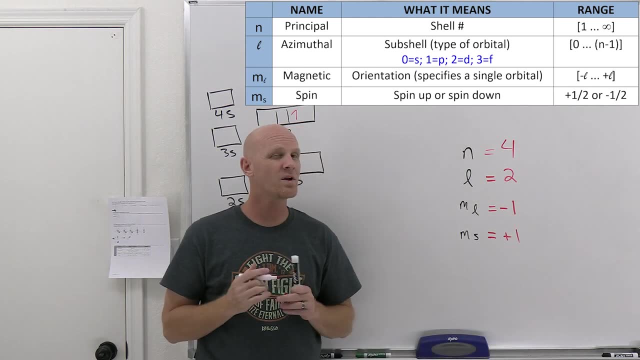 or plus 2.. Any of those would have been possible. And then, finally, for m sub s. so there's only two values possible. And so if I say, hey, what if it's plus 1?? Well, that's not one of the possible values. Again, the values for m sub s are either plus 1,